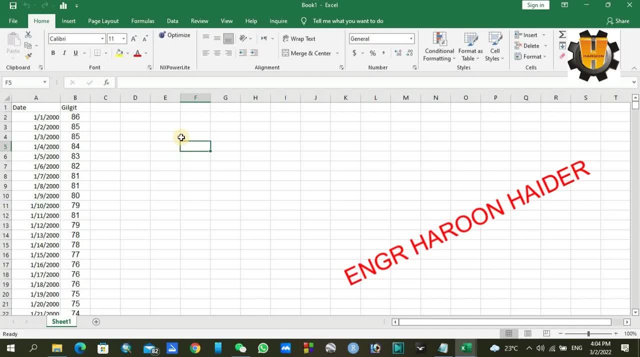 MODELS such as SWOT, QSWOT and others on monthly basis, So this data is on daily basis. We need to convert this data to monthly basis If we are working with the model- NETOLOGICAL MODEL- on monthly basis. similarly, if we are just using daily data, model is on setup on. 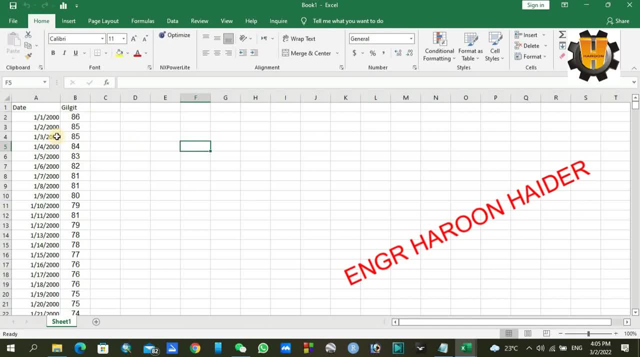 daily basis, So we need to use on daily basis. Actually, in my case, I have run the SWOTCAP, my AXSWAT software, on monthly basis, So I will first convert it to monthly data set. So how to convert daily data to monthly data? Just follow me step by step. So just select. 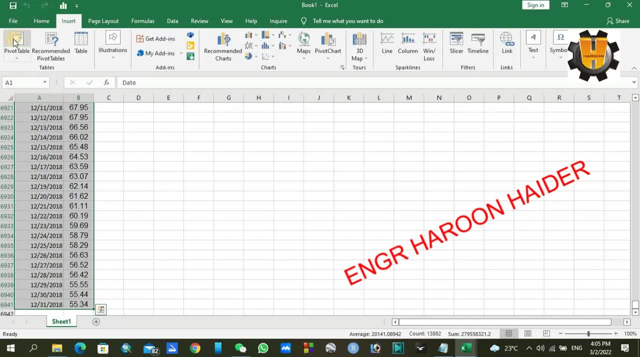 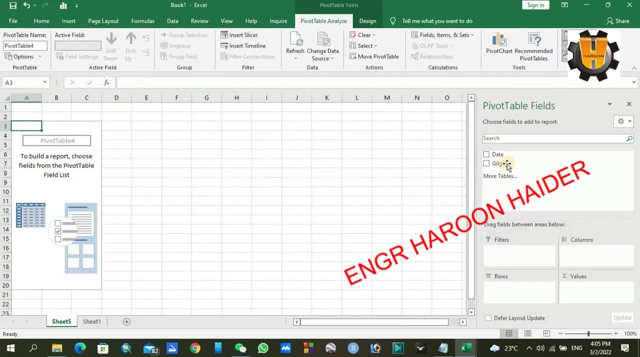 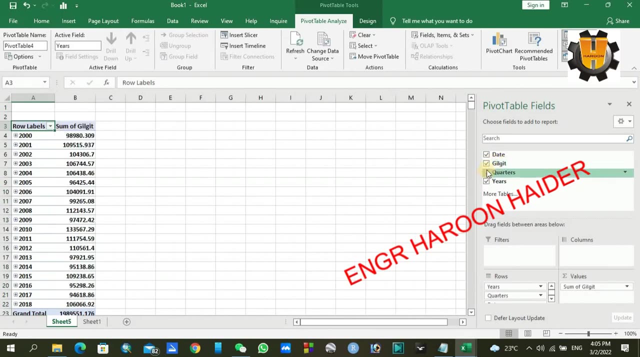 all this and go to INSERT tab Under PIVOT TABLE you will find in top left side. click on PIVOT TABLE and click on OK. So here you will click on DATE and on GILGATE, the second column, whichever you have, and 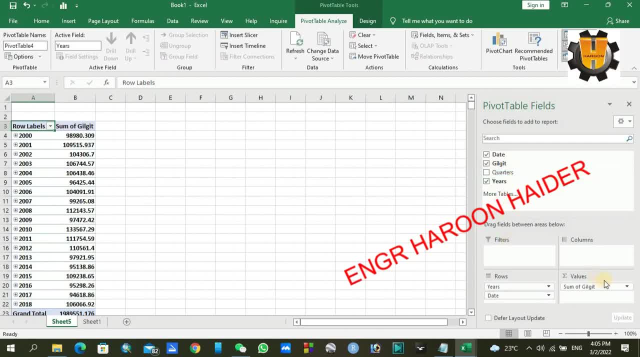 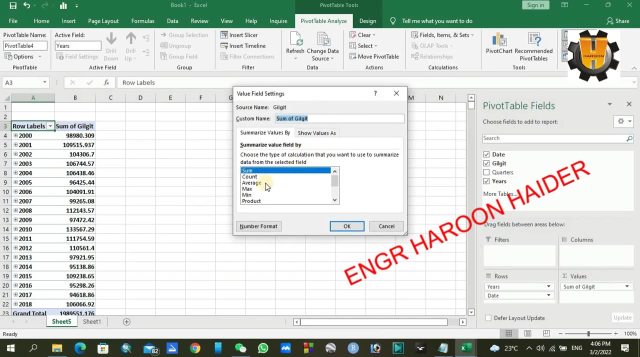 just uncheck this QUARTERS. Under the VALUES tab you can see SUM OF GILGATE. So left click here and click on VALUES. Under VALUE FIELD SETTING you have to check AVERAGE. So we are just going to use AVERAGE. 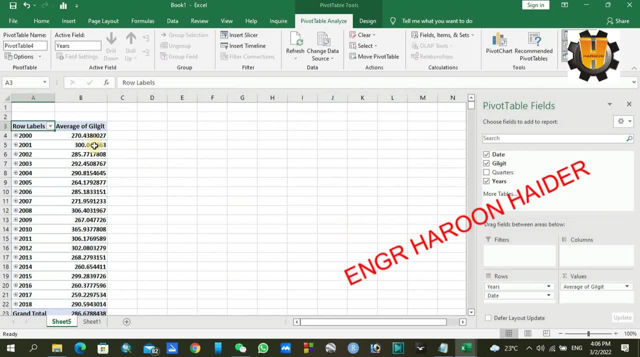 VALUES, not the SUM. So it is converted to 2000 and you can just right click, left click here, then right click and go to GROUP. So under GROUP SETTING you have to uncheck QUARTERS. So click on OK. You will see the data is starting from 2000 and on monthly basis. 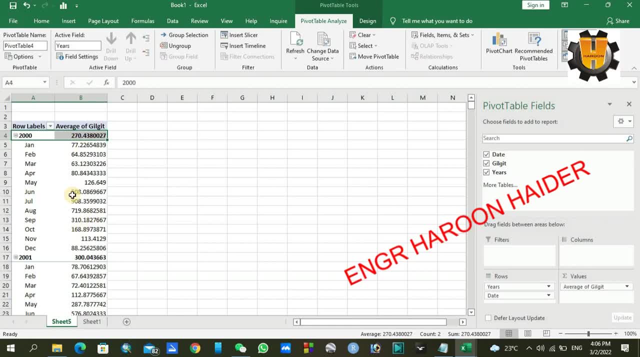 But here is the main problem. You can just copy and paste all these annual years one by one, or you can just use again right click and go to SUBDOTAL YEARS. Just uncheck it. If you uncheck it, it will be removed and your data will be returned on monthly basis. 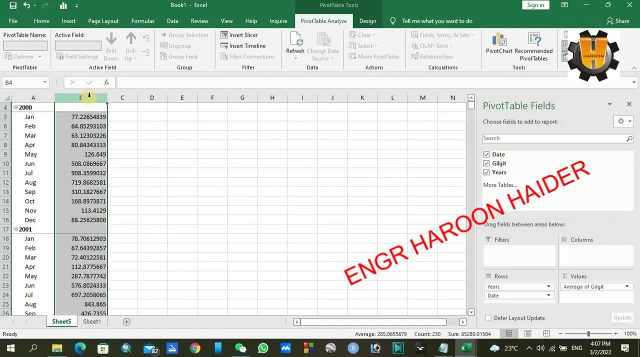 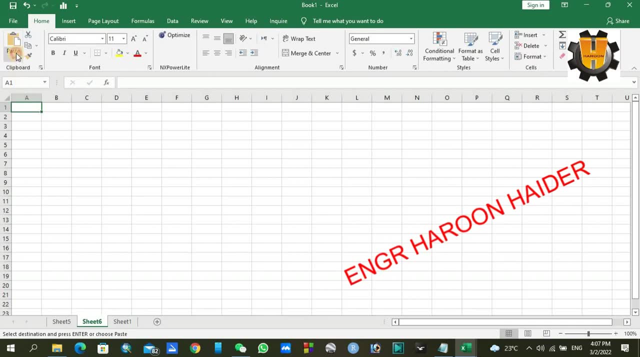 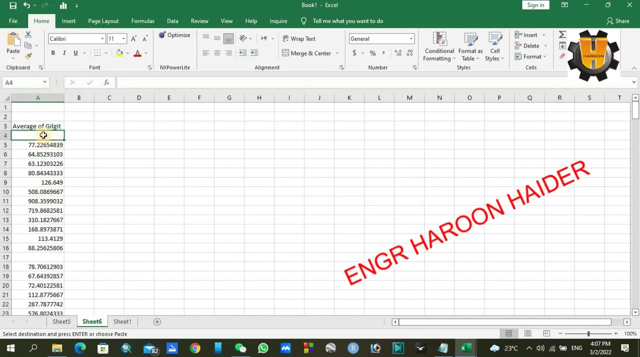 So just click up that column and copy. After copying, go to another sheet and paste it as it is. So here you can see the viewer, some values, some columns are blank, some cells are blank actually. So how to remove these blanks? just click check the select the table. I mean entire. 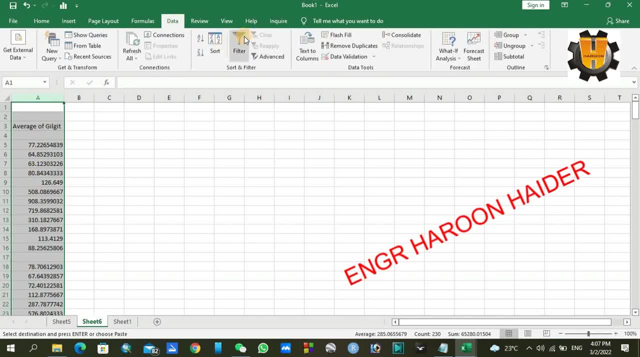 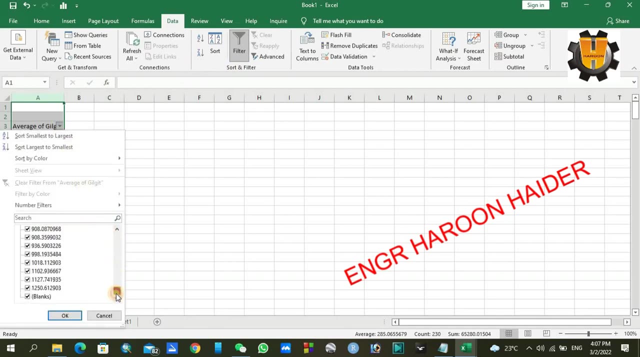 column and go on to DATA and again into FILTER. When you check FILTER you will see a down arrow here. just click down arrow and under the down arrow you can just go to the bottom and uncheck BLANKS. So in this way all your blanks value will be removed. 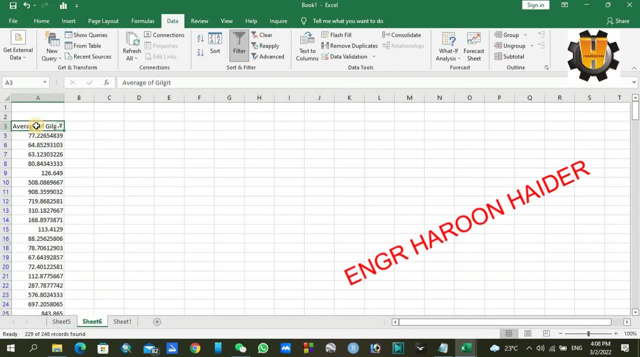 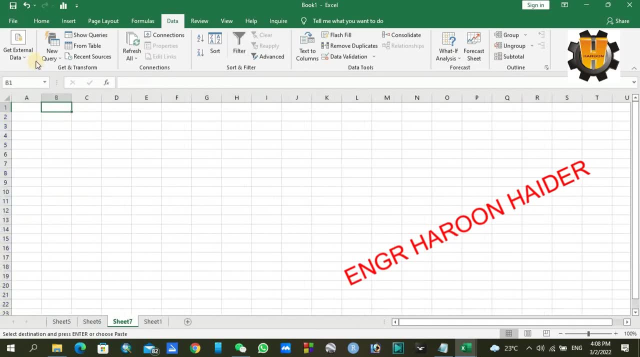 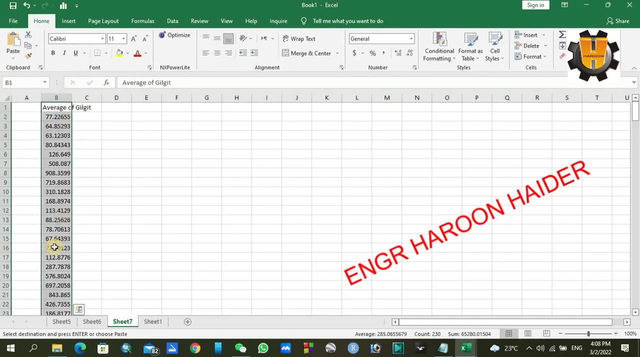 Again. you have to just copy this all CONTROL SHIFT DOWN ARROW and you will copy CONTROL C and go to NEXT SHEET. So here you can use PASTE so you can see the. your data is already pasted here, okay. 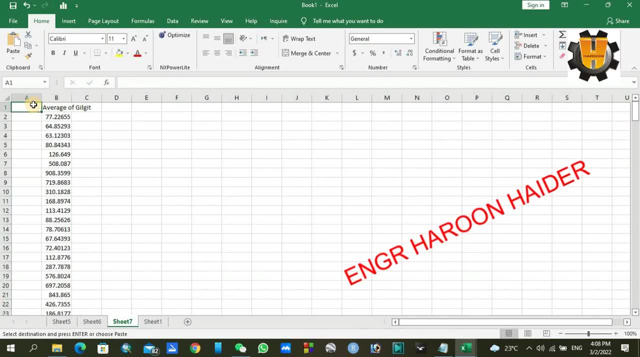 But here there is no DATE column, we will just write it as DATE. so it is 1st of January. starting month is 1st of January 2000,. sorry, January. you can write as January 19,. sorry. 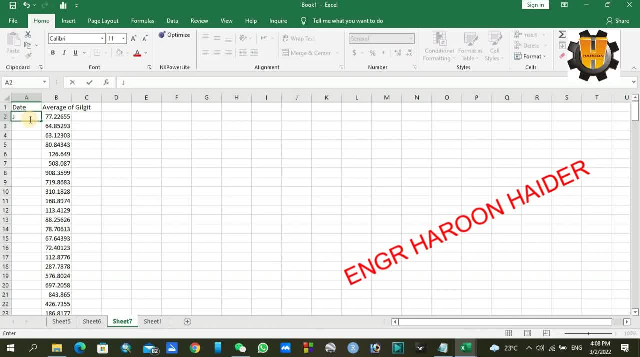 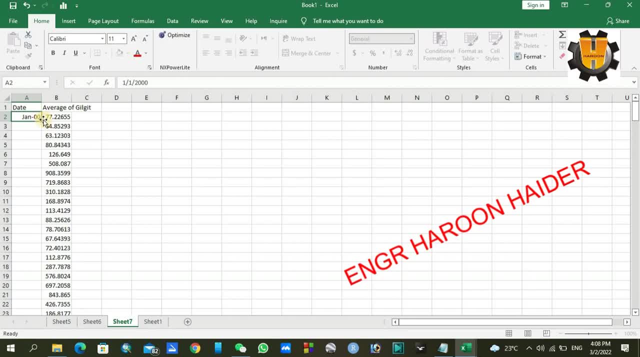 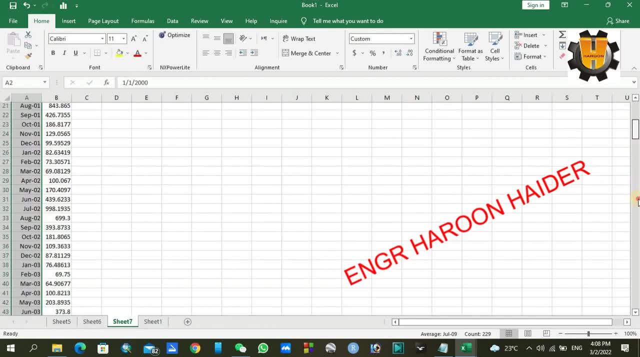 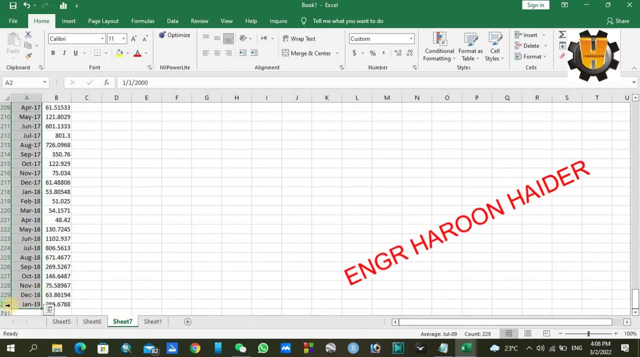 So you can see you're delete and it is SEPTEMBER 18, one extra column there and we can just remove it. ok, Let me go to start again. you need to convert all DATA, so just delete the last one, because we are just working on some variety now. still there. 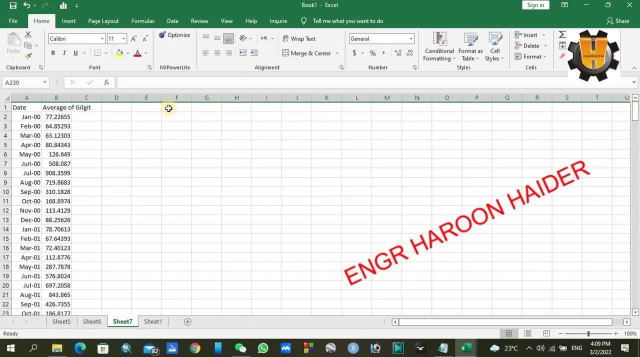 is something we have to. we use other things. let me show you. we have to add some. you can see here a test. put the dash here, extend it to the end. okay, now we have to add ID, so ID can type ID and from here we can start. 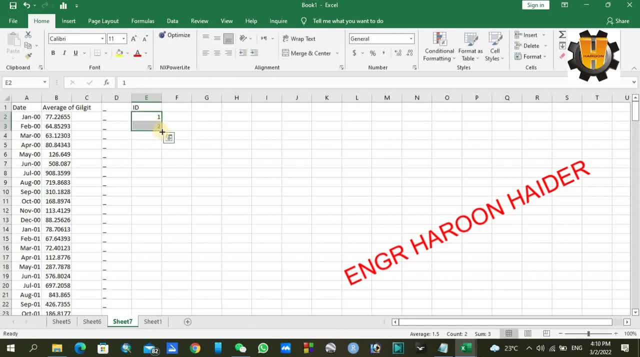 with one ID and from here we can start with one. okay, and after ID we have to add a month and year, so just it's months, okay, so first one should be the first month, or just use equal sign and type month the date column and enter okay, in this way you are all the months will be. 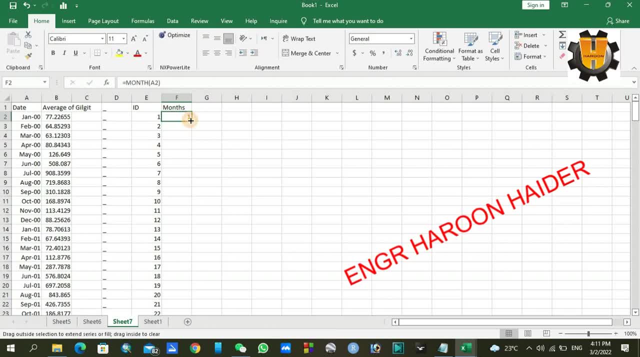 extracted from date column. so just double click and it will be arranged. okay, then we have to add years again. similar method is equal sign year and the first one and check the date column enter so it is year option. again, just double click here so all the years will be extracted: months, years and. 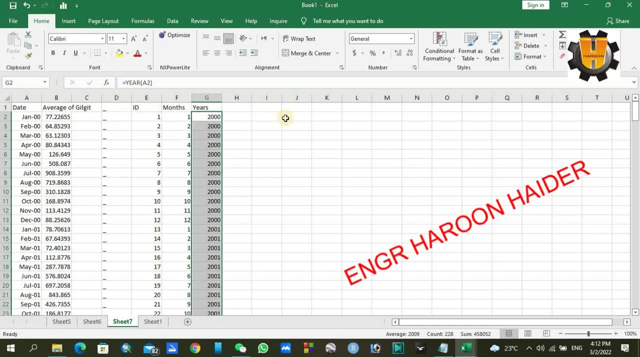 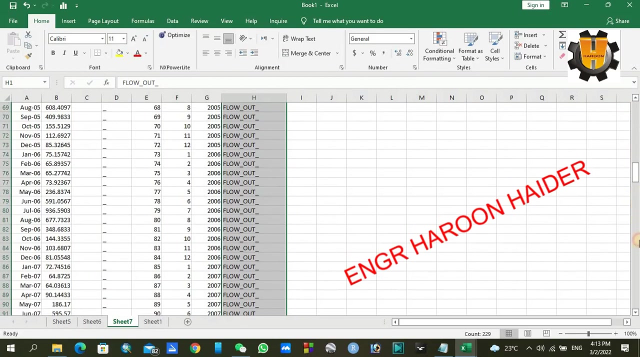 ID and just say dash symbol. so now we have to merge all these. one more thing: we have to write flow out, flow out, flow out. and ok, let's type this one and so you can see: flow out till end. now you can see them, this flow till end. okay, now the next one. next is to join all these, so for 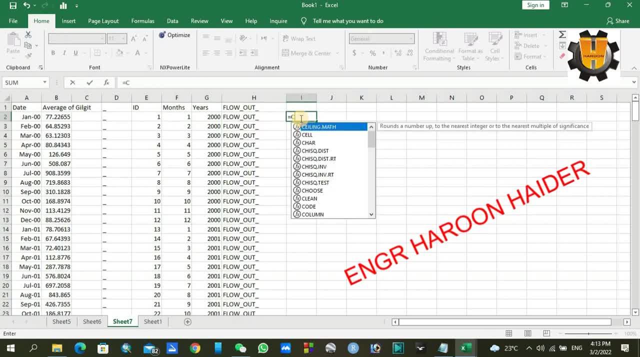 joining, we will use equal sign c o n, concatenate the first one, double-click, and we have to merge all these in a proper way. let's see float comma, month and here okay. so flow one, two thousand and close the bracket and press enter so you can see: oh, there is an error. I'm gonna go again because we have to add a. 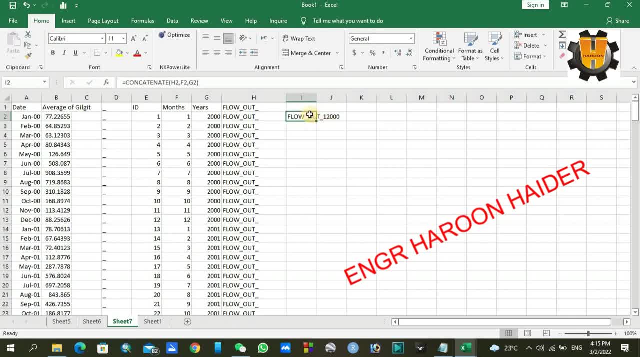 dash symbol after the month two. so I have missed that. just again repeat and upload and month, and again we have to use this one dash comma and that. so now it is fine, let's see, yes, it is looking great. load one, 2,000 and just need to. 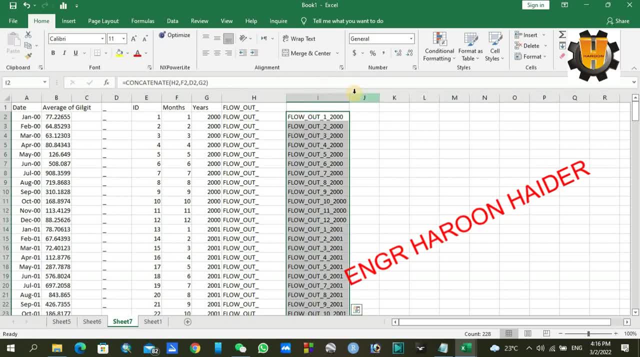 typically can go to end: okay, so it is our float and similarly, here is our, our fellows copy it and paste it in front of it. okay, so in this way you can prepare your data for calibration and in the same way you can prepare your data for validation. just, 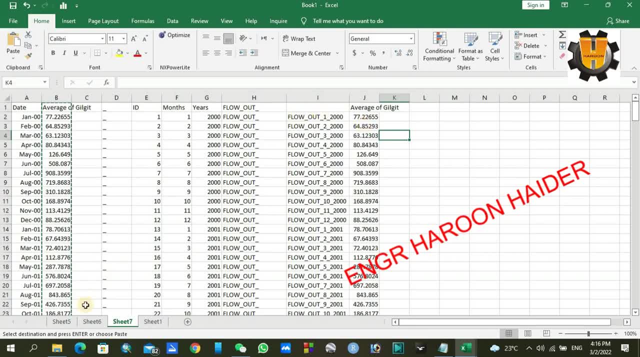 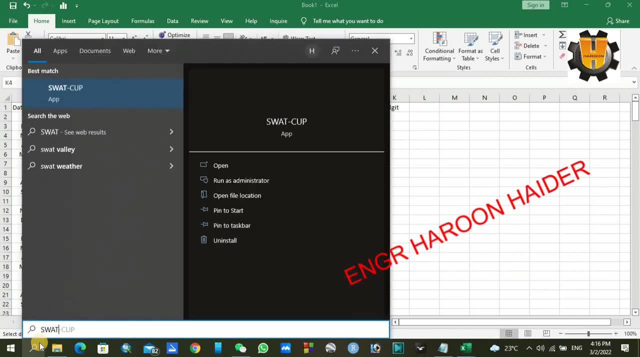 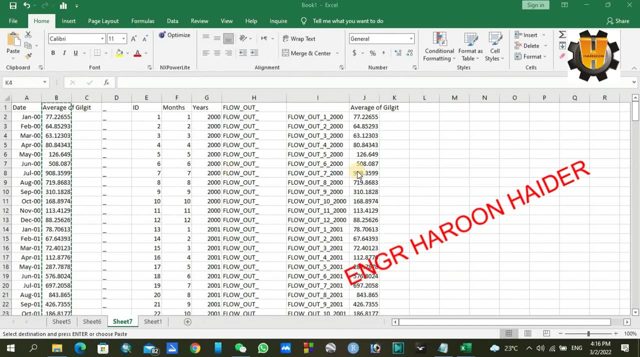 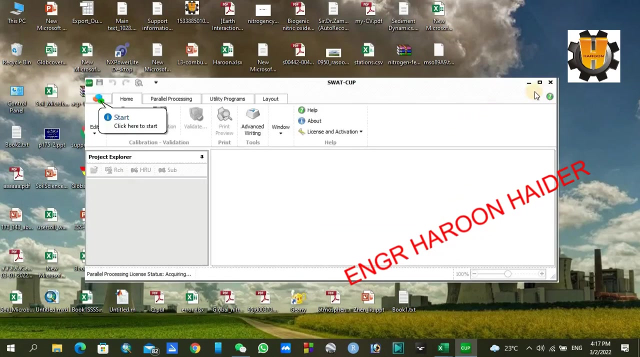 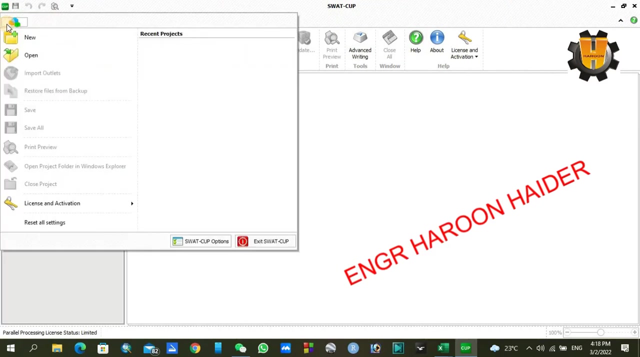 you need to. I will show for the steps after the in the SWOT cup. let's say: we can with SWOT cup. let's open cup F and open it. let's see, okay, SWOT cup is opened and we need to click here to start new one. 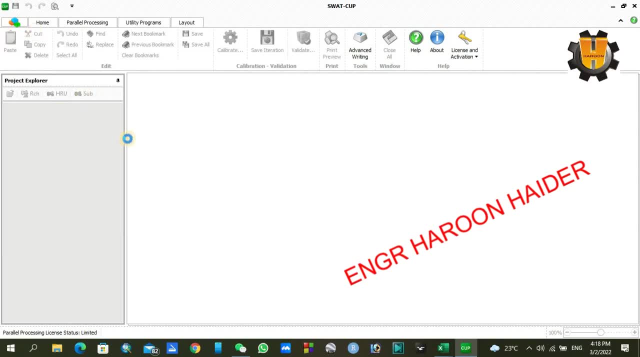 next, it is asking for text in out location. so it will be located where you have run your ArcSWOT or QSWOT model. so it will be located where you have run your ArcSWOT or QSWOT model. so it will be located where you have run your ArcSWOT or QSWOT model. 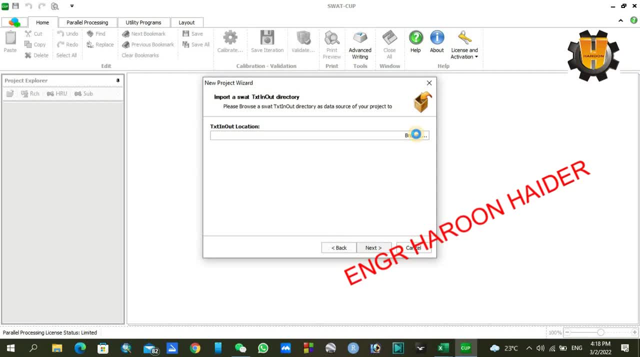 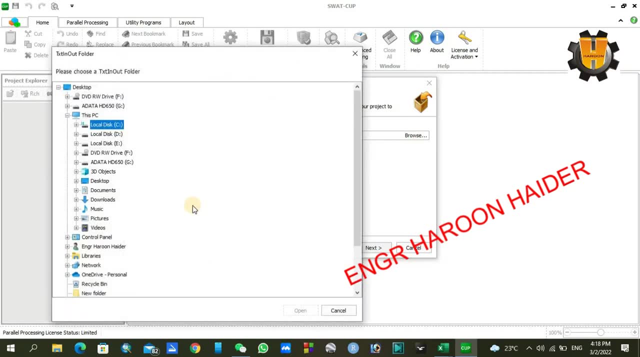 so I am just going to give it my text in our location and just click on browse. it will move toward your directories. my project is located under my data. find folder 3 here and scenarios and the zero year skip and here text in our, so in your working. 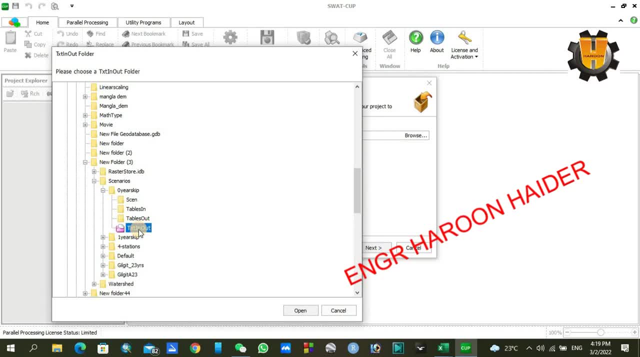 directory in which you have run your SWOT cup or, sorry, our ArcSWOT or QSWOT model. there is a folder of scenarios. under scenario tab you will find the default values, or you have your own, maybe another. so under scenarios, go to your folder- default folder- and click on. 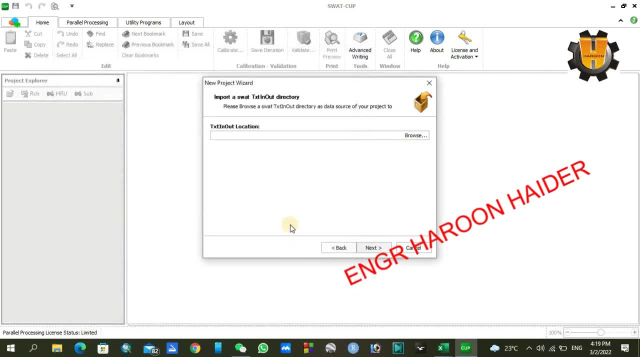 text note and so I have you in it, my textino directory. just click on next. so it is asking for SWOT version. I'll see my SWOT works on 12, so you may be yourself make very depending upon your first. you have to give you a SWOT version. 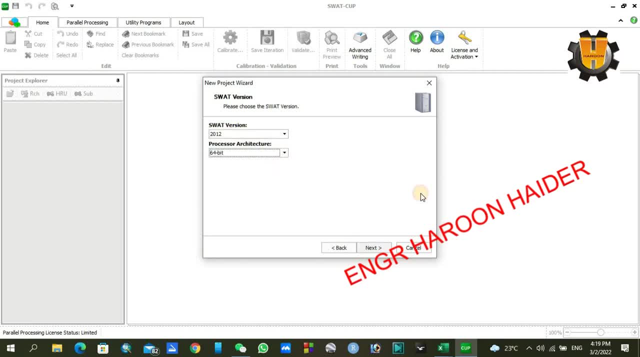 so that's that. mine is 64-bit. so next and choose a project. in the project type you have to choose Sufi tool and click on next. so project name, where you in the new project name you are working on Swat Cup name. so I'm just giving it to my name. 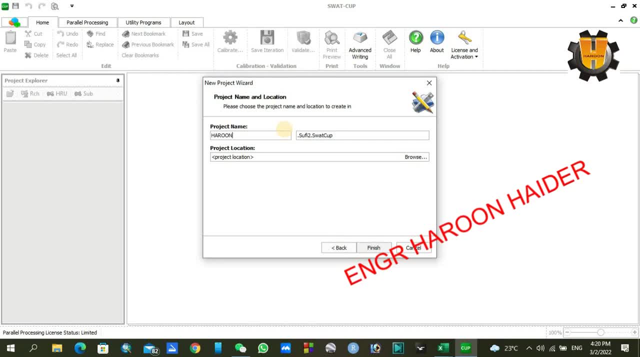 I can see. okay, so for the application, let's browse where you want to say: this is the name you want to give, the location you are very want to say. so I'm just going to say with them documents and finish. so now it will start copying from some files, from your text in your 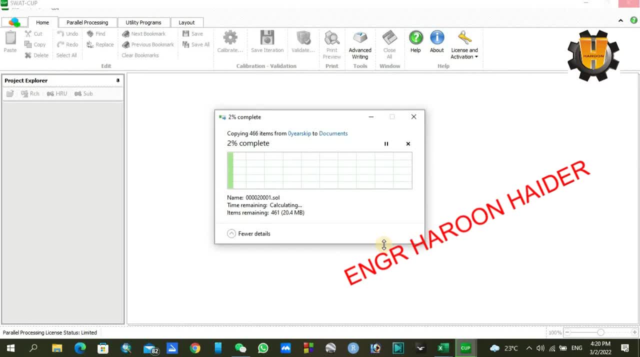 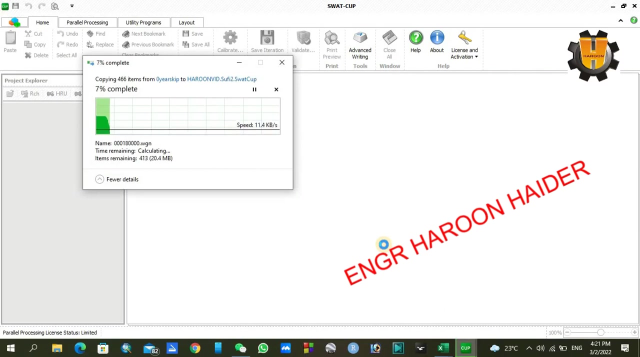 files from your project to Swat Cup. so it will take some time to finally submit it so you can see in the page of files who are copying from Swat Cup. so 10 expiration date, which is 31th January. so I have copied it and some other stats are also copying. I have to wait. we will wait till it. type in Swat Cup box, click on the drop down menu. then until it writes it will stay inoppy in Swat Cup. so this is Swat Cup, the чтоб 123.00. so finally, I am going back open up on the website. so the job that I have created. so let's do that. I will just copy theJSY to Swat Cup. so how this happens. we have finally got the Swat Cup. I have seen that the SKU in Swat Cup available. let me just put opposite to the magic file you want to copy, then continuing to copy. 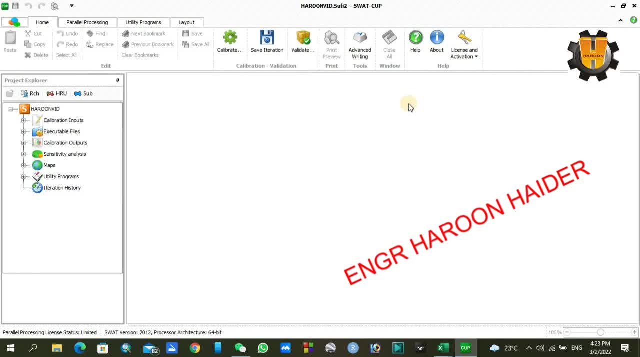 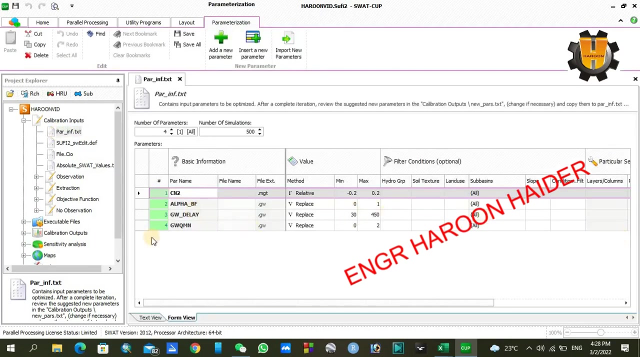 Okay, after the copying will be completed, you will see your project name here. so go to configuration inputs. so under configuration input you have to find the parameter informationtxt. so double click. we will find some parameters here, four parameters. so these are some basic parameters. these are not enough. it is only the game of some parameters actually. 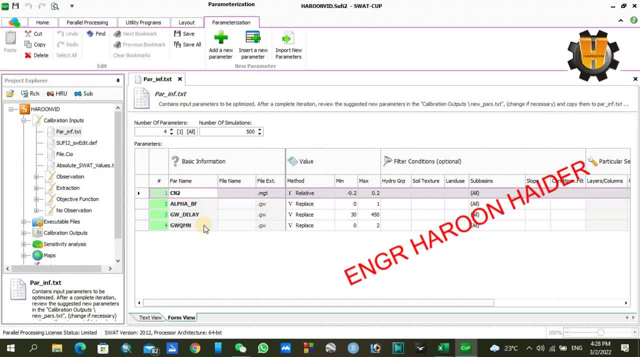 so we have to use different parameters depending upon the characteristics of our watershed. so in case of gilgit river, albeit so, I will use 22 parameters I will discuss here one by one. so first, CN2 is a minimum. well, you should be minus 2.4. 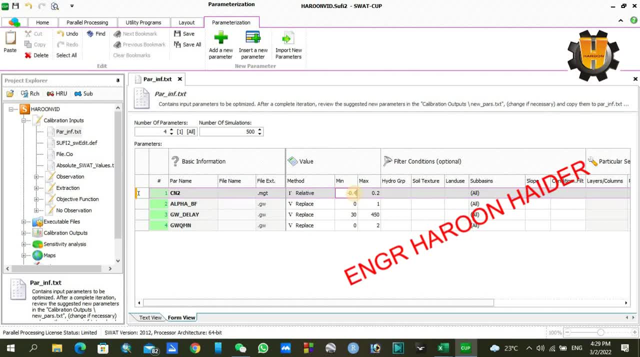 so you can use the same values as I am providing for your watershed 2 if it is on mountainous or the snowy watershed watershed. so for alpha bf it is from starting from 0 to 0.06. i have got these values after sensitivity analysis. i'm not going to discuss sensitivity analysis here, i'm just going to add. 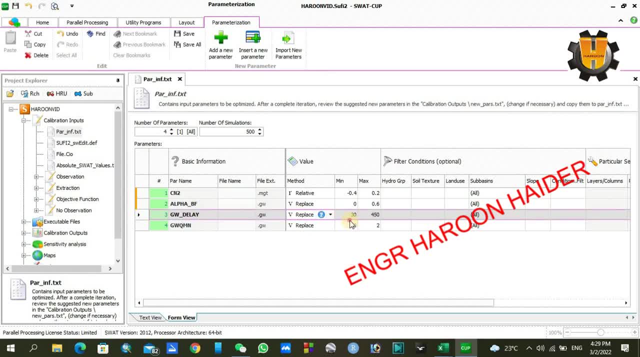 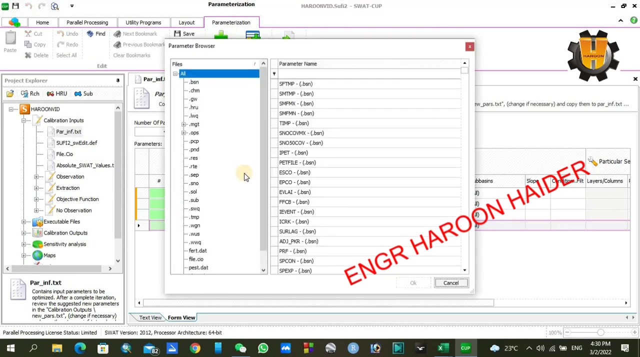 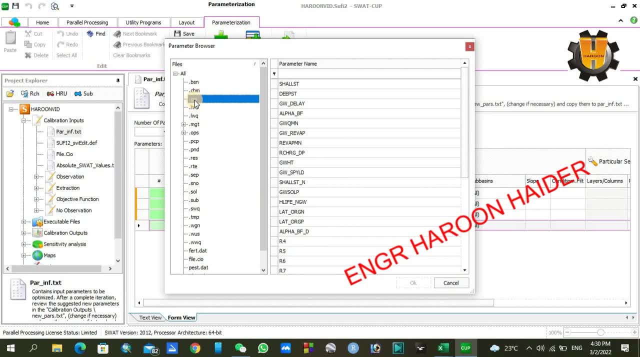 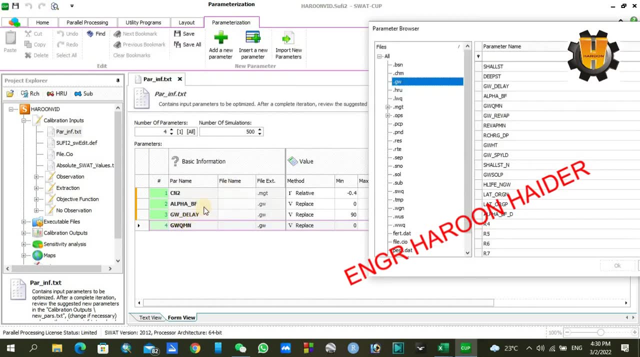 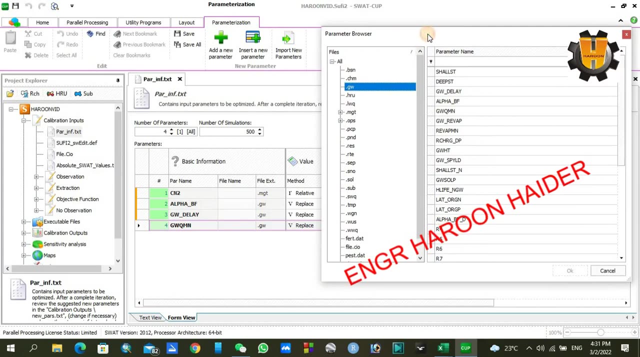 in dasaw you can find i have already uploaded some groundwater parameters. let's see, that's. that's gwm and gwa daily and all our groundwater parameters. so we have to add some other gw parameters such as w, rev and dp. so the gw session is ready here, okay. 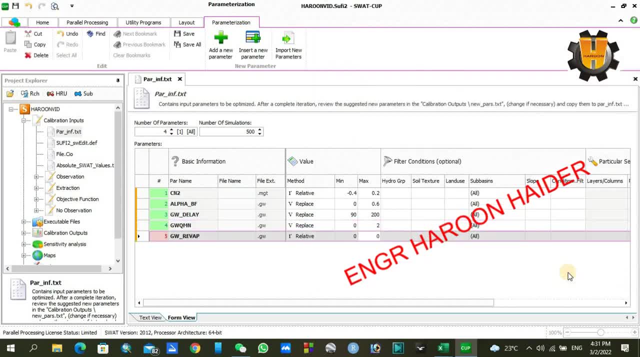 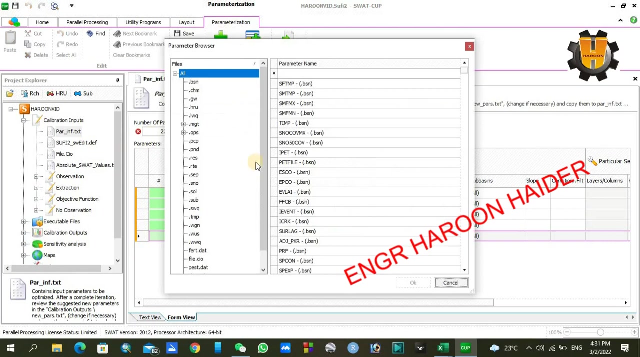 jags to the web. its value should be zero to zero, point two. okay, okay, so it is looking at the red. so if you have to change the number of parameters from here, so it is green, so I am, we will use 22 parameters. now we have to add some other parameters again- GW, so it is some time. 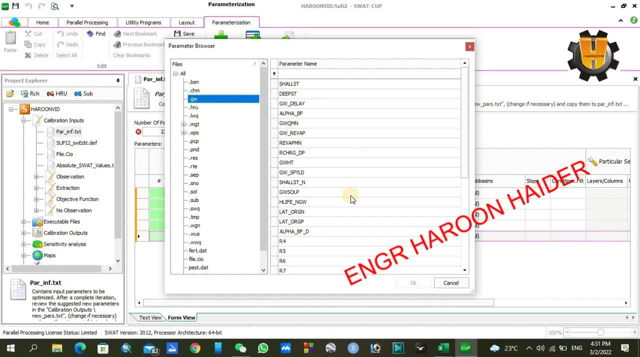 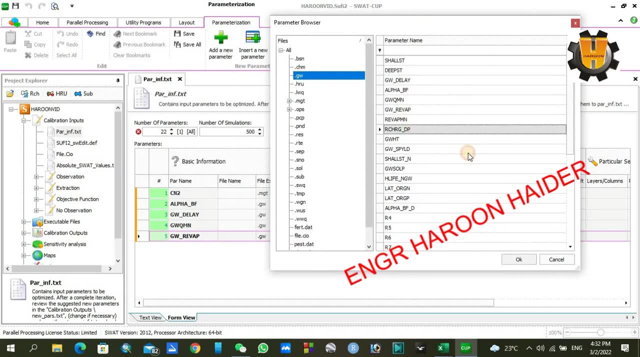 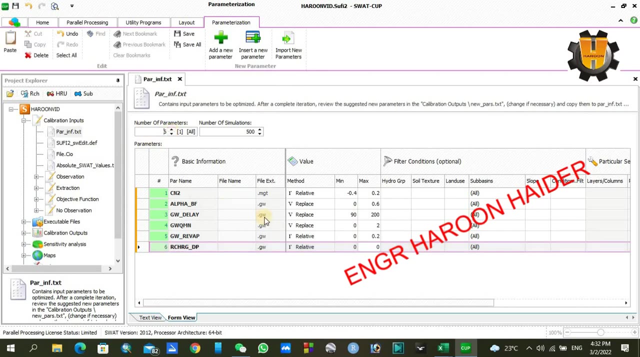 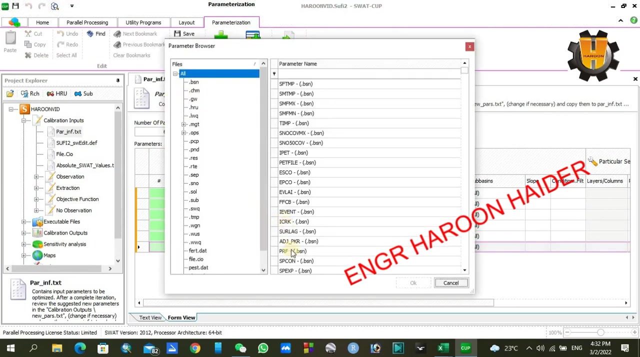 taking work, you can. you have to select one by one. again, I'm going to use recharge deep recharge, okay, so again six. so recharge deep value should be zero. from 0 to 1. okay, and again one new parameters, RT parameters, so it is see it. and two, and similarly see it, k2. okay, so these values, their values should. 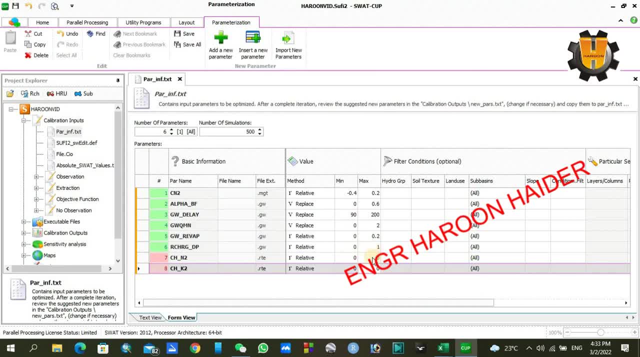 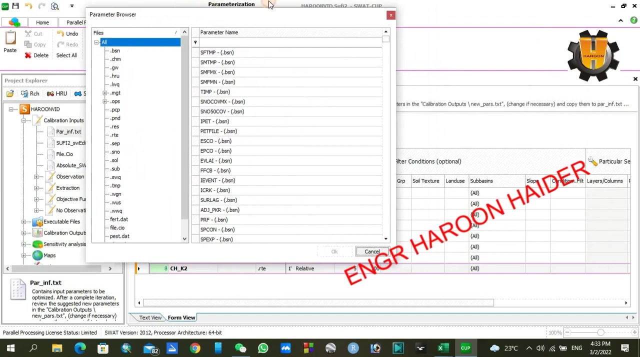 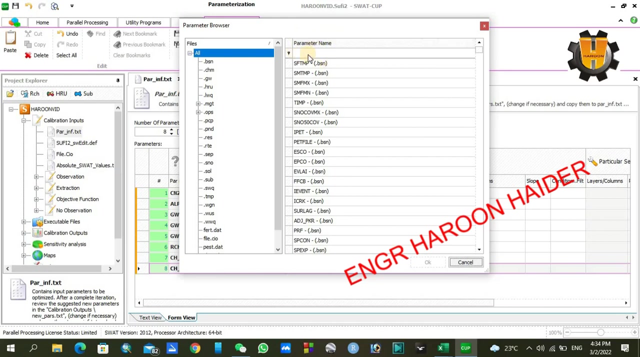 be from 0 to 0.3 and 5 to 100. these values I got using some uncertainty analysis. I'm just repeating that, those steps and adding those values which I started, initial values. so again, again, RT, it is some alpha bank and okay, and it said it's where it should. 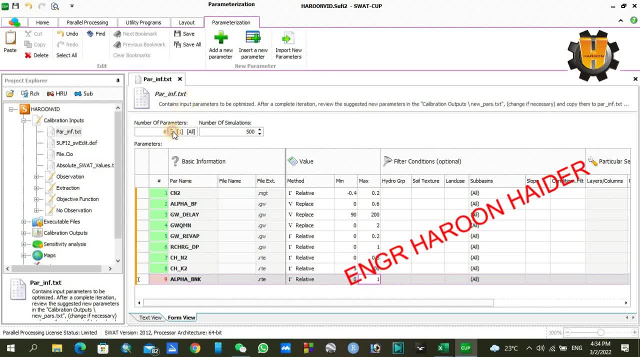 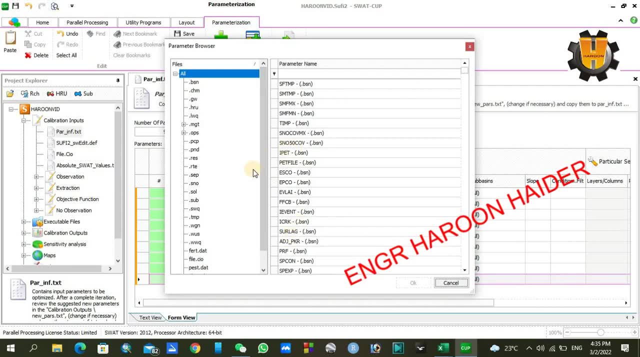 be 0 to 1. so again a new parameter, some as well parameters. we have to find this one saw the AWC available water content, okay. so again RT, it is some alpha bank and okay, and it said its value should be zero to 1.. 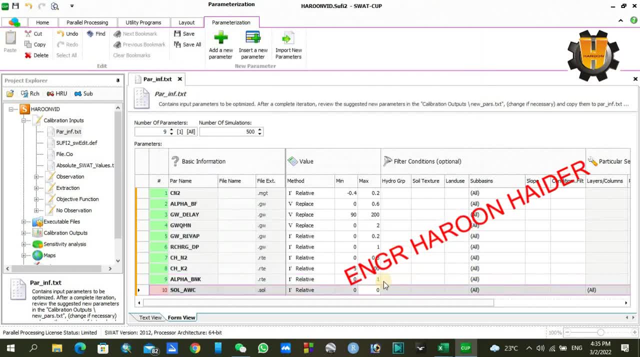 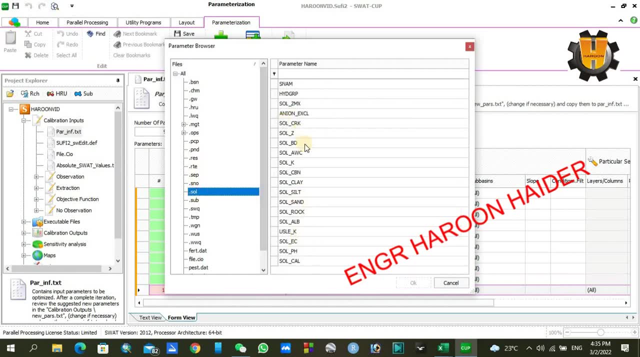 we have to find this one, okay. so again a new parameter, Sol parameter, Sol WC, Sol K here and similarly add a new parameter of Sol N. maybe we have missed Sol BD. bullet test is also very important, so I'm just going to use Sol BD square. is Sol? again, need to check. 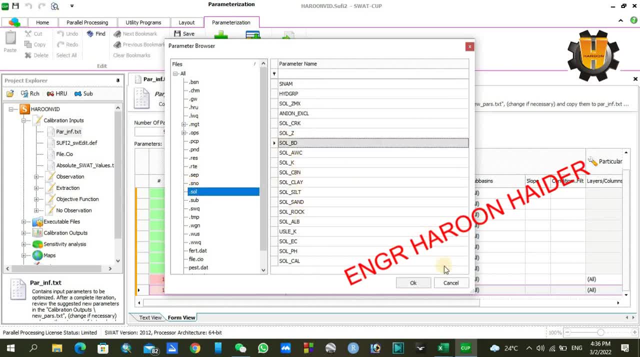 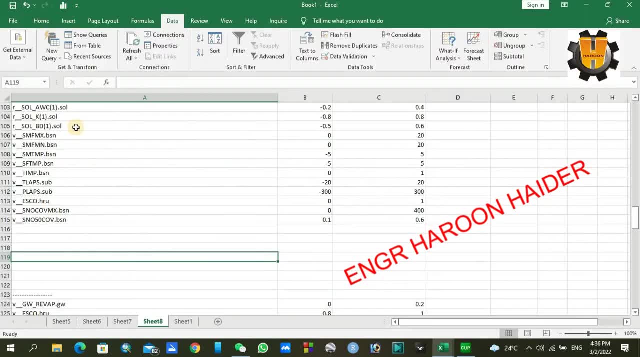 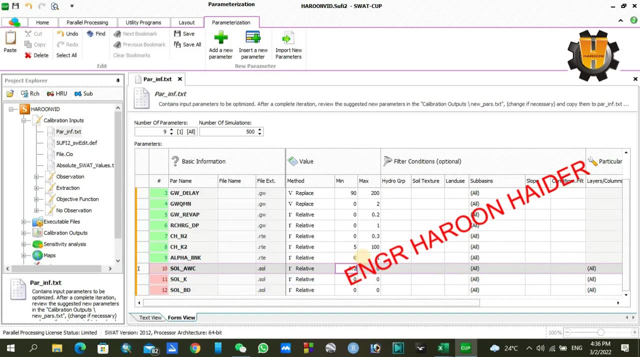 and where is Sol BD? this one, okay. so we did not provide any values here. we have to add values, so its value should be minus 0.2 to 0.4. okay, and Sol K value will be minus 0.2, 0.8 to plus 0.8, and similarly Sol BD. 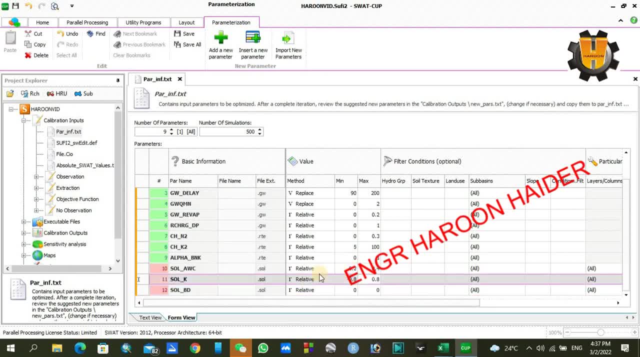 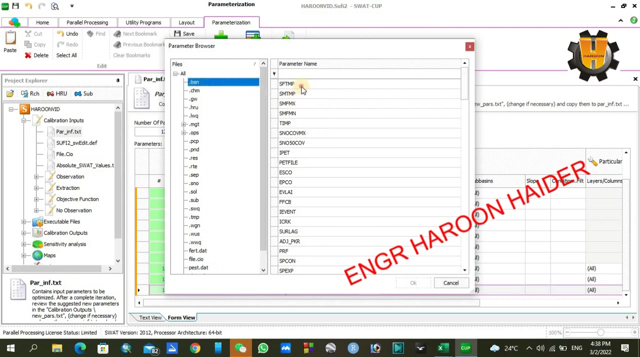 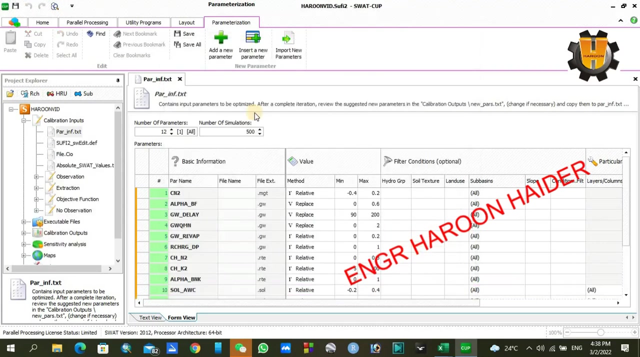 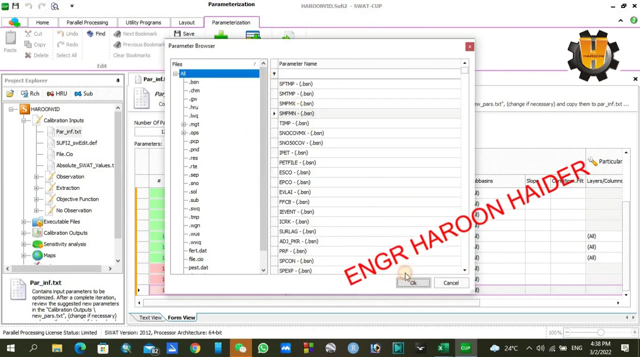 Sol bulk density. its value should be minus 0.5 to 0.6. okay, so we have again new parameter. so here some basin base parameter: SM-SFTMP, and similarly SM-SFTMP and SM-SMX and the it is first2, so SM-SAFN. so these values, the value should be: 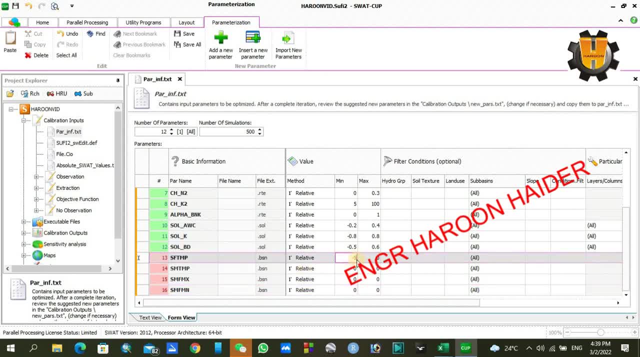 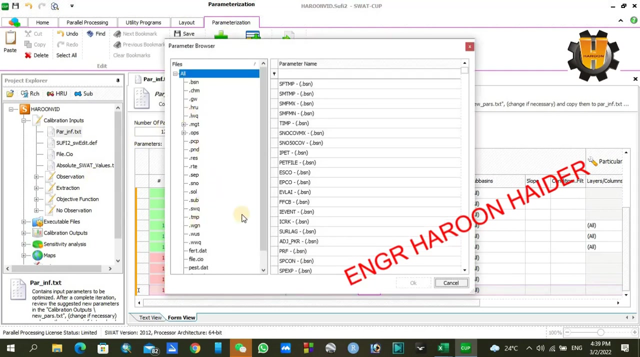 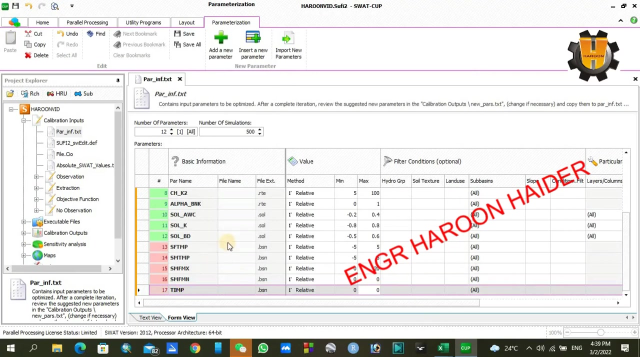 minus 5, 2-5, and similarly minus 5 to plus 5, and here FMX set should be 0 to 20. okay, stay, some parameters are left again. add parameter Besson and this and we have to go to find the TMP. okay, so the empty values should be. 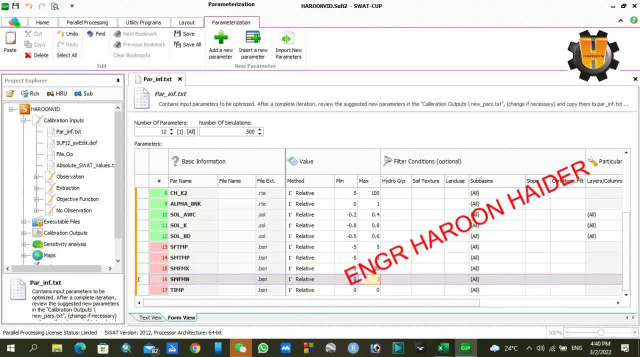 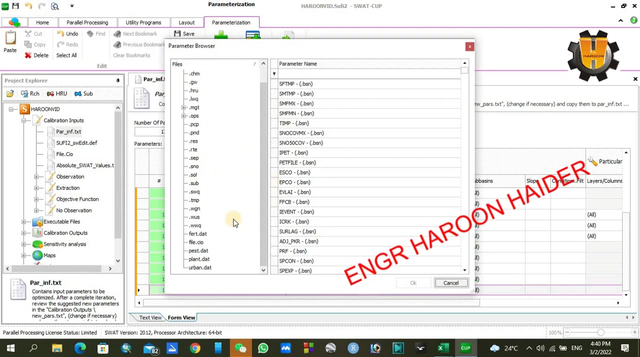 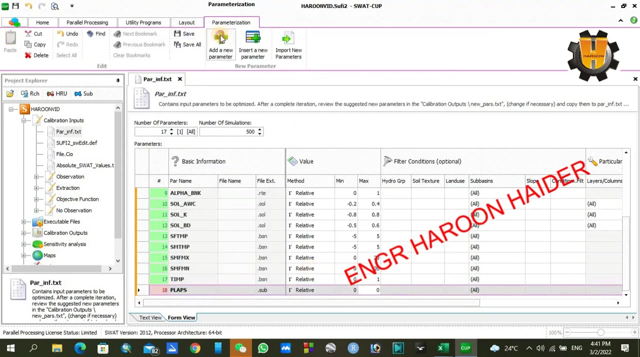 as some FMN values in which 0 to 20 and the empty values should be 0 to 1. okay, we can just increase and add a new parameter. I can find some submission parameters, CB and the submission P laps, and okay, similarly, again, submission and P laps. 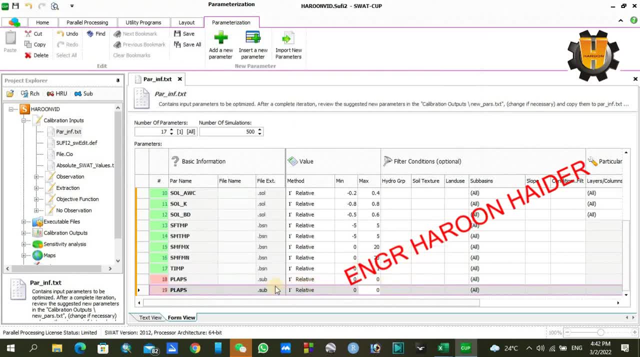 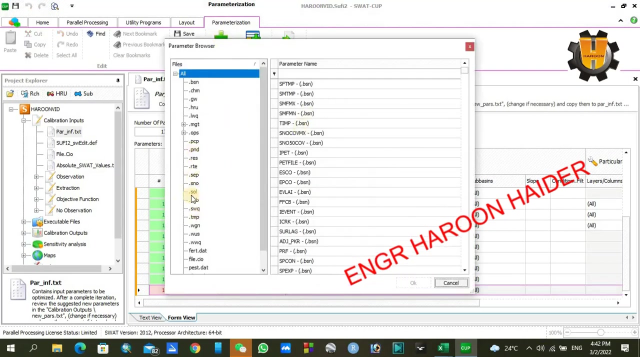 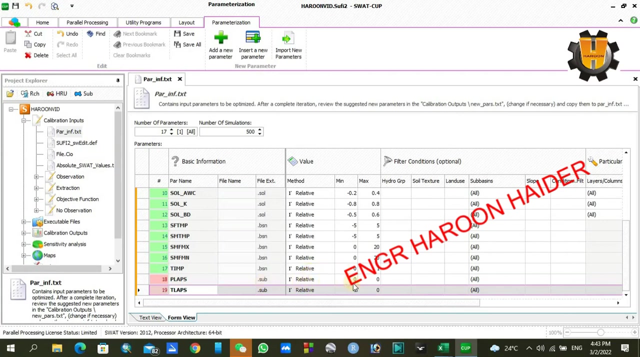 so so T laps- and I think I have repeated T laps again. so just clear and delete it. okay again, add a parameter submission and here we can find: okay, T laps, okay, and the parameter: T laps should be minus 20 to plus 20 and for T laps it should be minus 300. 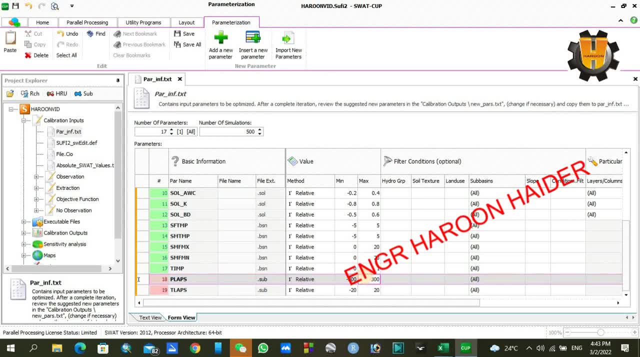 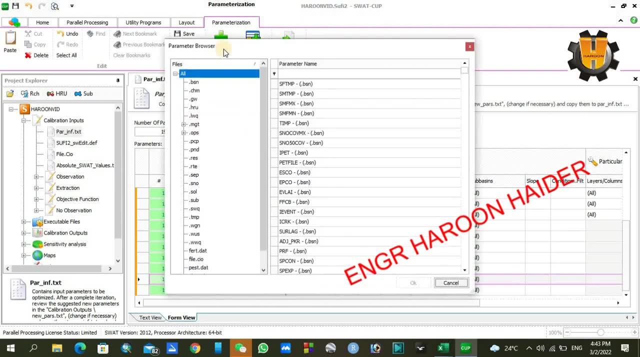 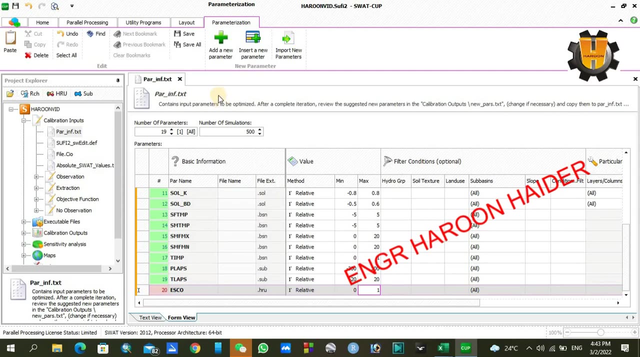 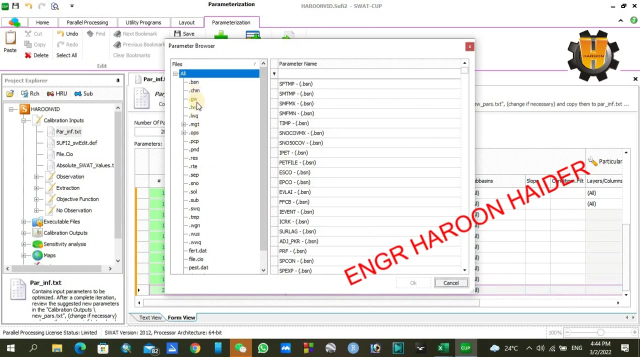 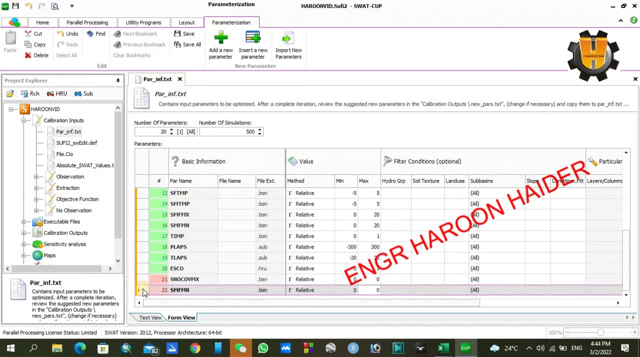 okay, okay. so now okay, another parameter, another parameter. I tell you 0 to 1 and add a new parameter. so Besson SNOMAX and Besson SNOMAX, okay, so I can just repeat it again. so I will delete this SNOMAXIMUM. 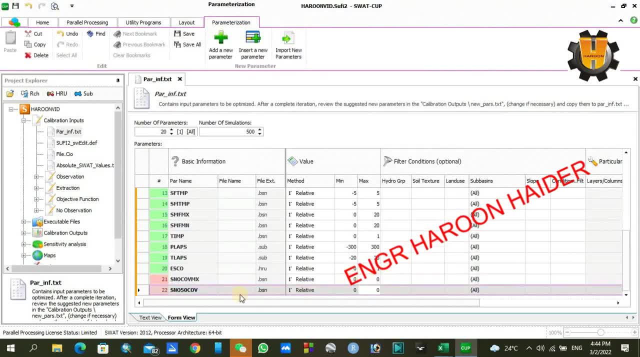 and then SNOWFIFTYCOVER. okay, so SNOMAXIMUM, which is 0 to 400, and then SNOWFIFTYCOVER, which is 0.1, 0.1 to 0.6. okay, so our 12.5 have this left it. 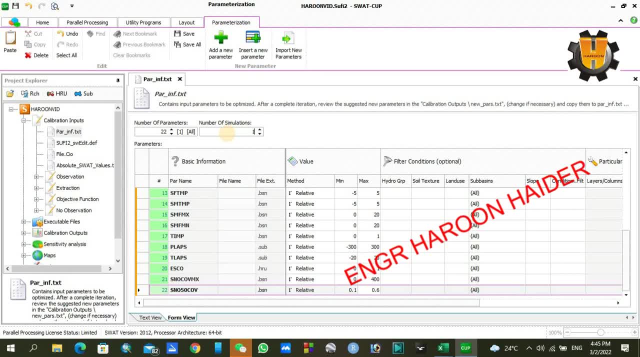 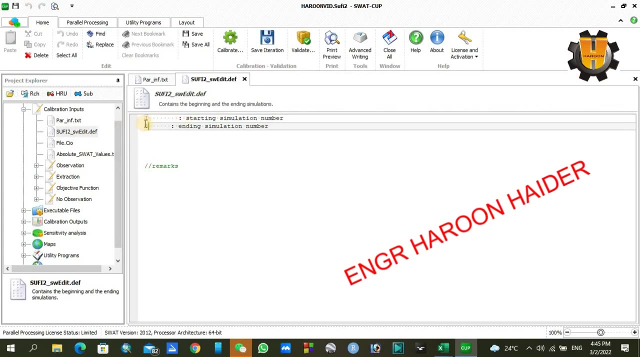 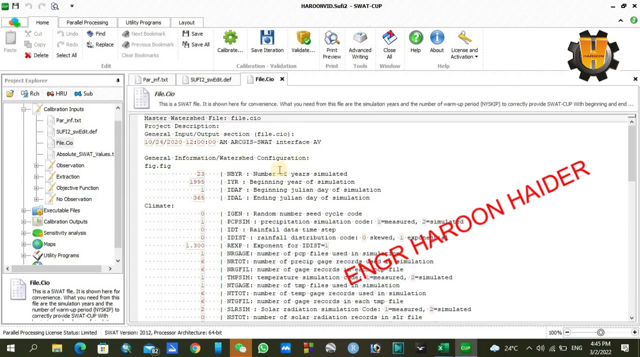 number of submission. have 1000 submission for each step. so first step is done under C2, starting submission 1 and ending submission should be 1000. okay, and file is CIO. ok, you need to change this number of year according to your distribution. so i am changing 23. my total year: 23 years from 1995 to 2017. 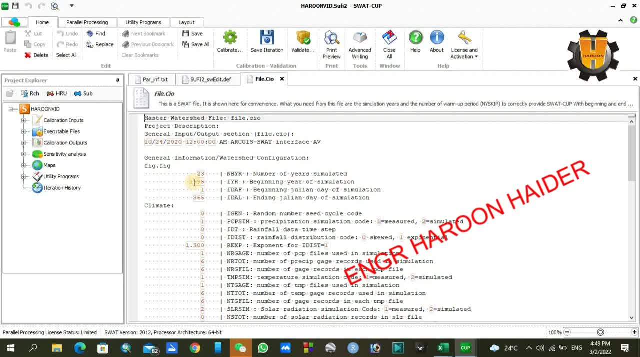 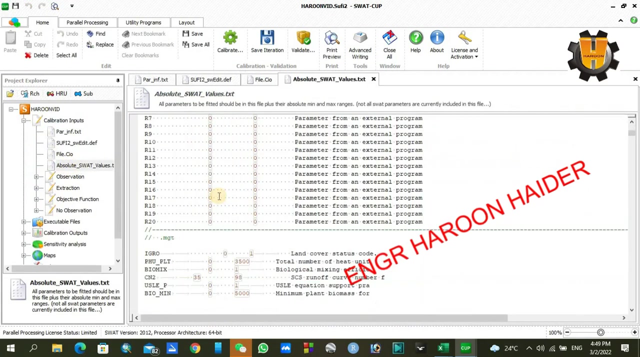 but i have to use 12 year for my calibration and remaining 11 years for my meditation. so i am just decreasing it with 12, so my starting year is 1995 and beginning year is 2021. so next step: select smart values. just keep it as it is. 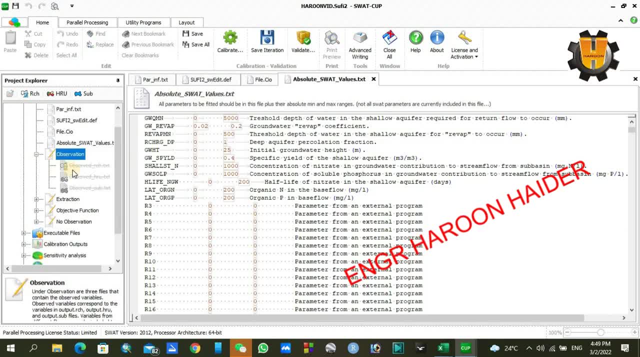 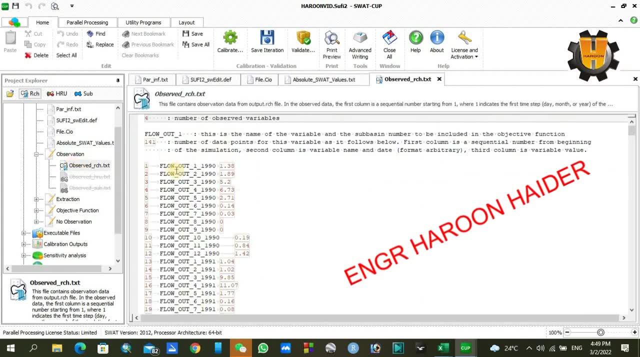 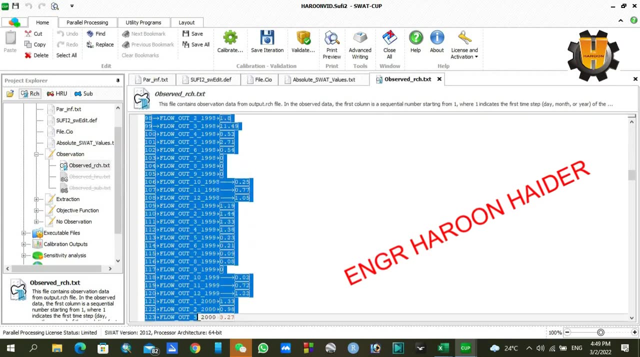 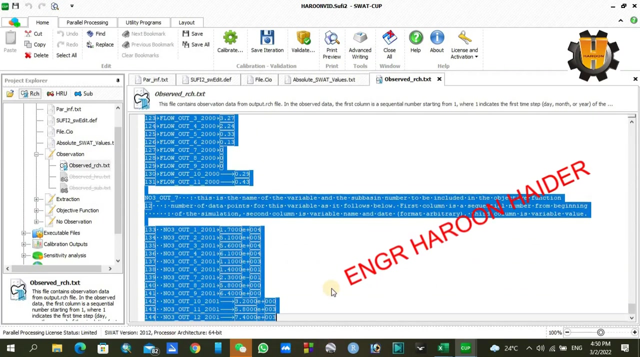 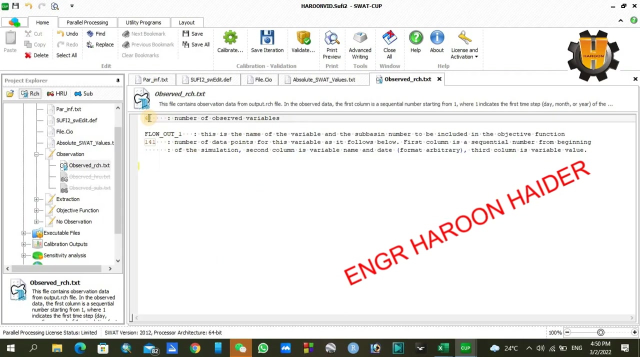 click on observation, click on rch and observe rch, so it will help delete all this data from here to end. so this data is already in default data set and we have to provide our. so number of observed variable will be 1. so that is only. 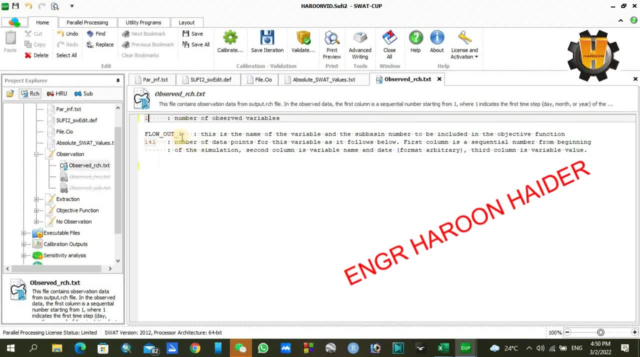 ok, and so here it is working as load dash 1. so here you have to provide the last load of your last submission submission. so i think you have, if you know the number of submission in uber, rswat, rswat or qswat project. 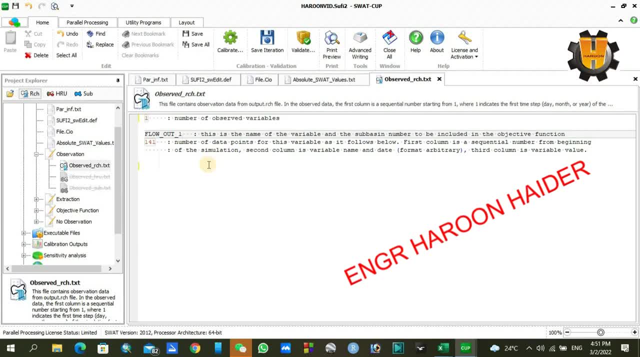 so in my case this is r27. yes, so just change it to this same and the calibration i am using for 12 years. so 12 years have 144 months, so just type 144. and now and now, here we have to provide our observed data sets. 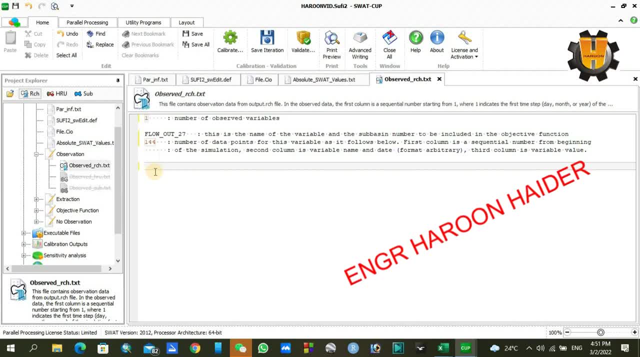 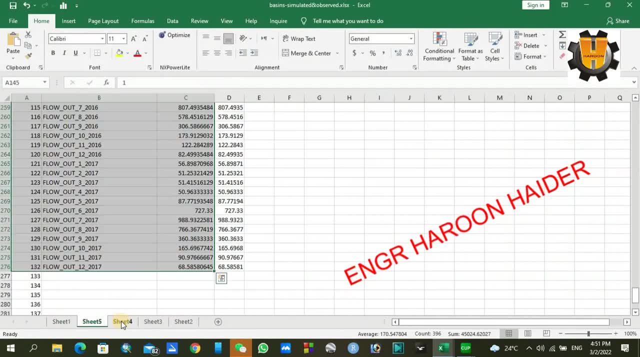 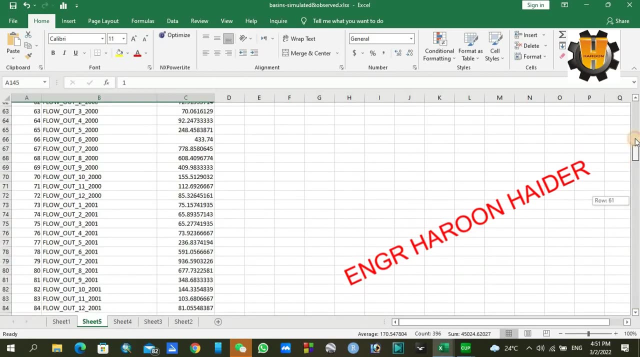 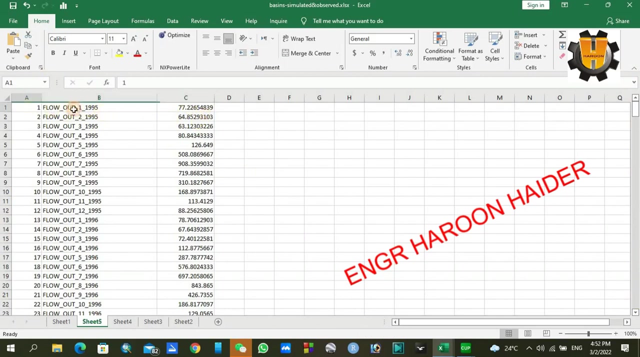 so we have already prepared. i already showed you so here. lets see. so from here we can recover data sets. first one is id and some of the other one, and at the end is our average flows. so we have to copy 144 ratings here. ok, from until 144. 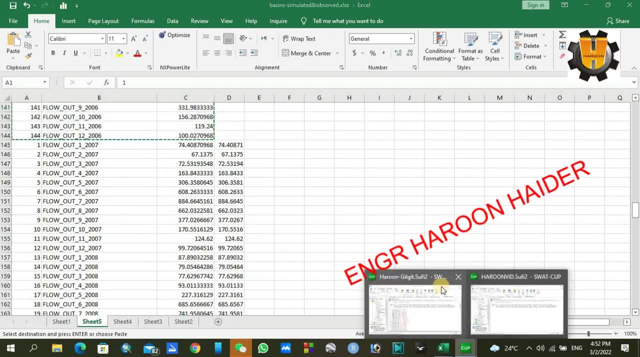 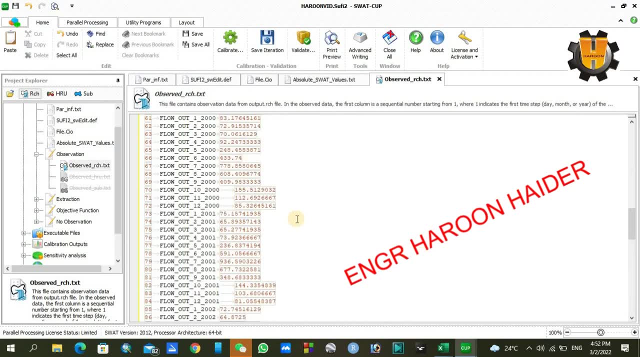 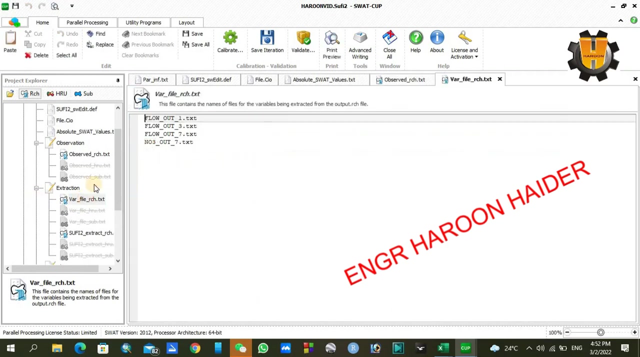 ctrl and c, copy it and just go to rswat club and paste it. so job is already done, so data is already pasted. ok, so now go to extraction variable file dot, rch. delete all these and just add 27, the last submission value at the end. 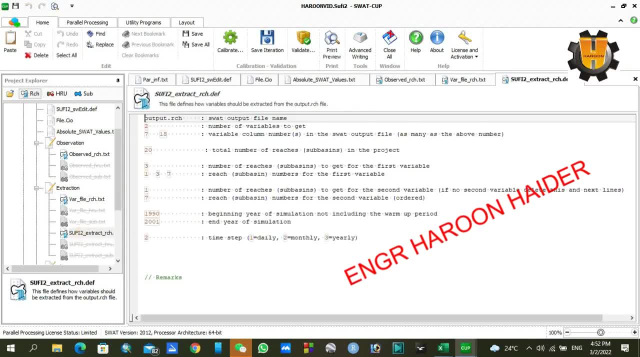 so if you do extract dot rch, so number of variable to get 1, and it is 7th. 7th column is for flow, so delete the other one and total number of variables is 27. now we have to find the last subpression. 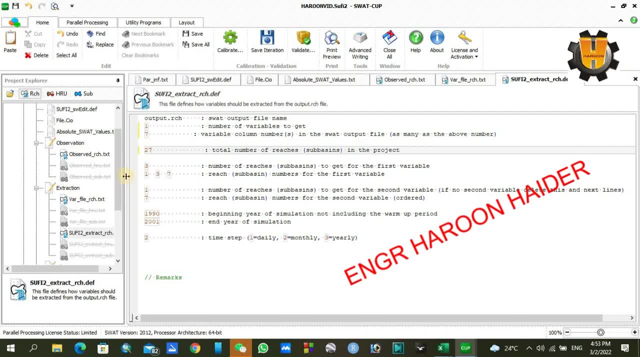 so we have to find the last subpression. so how many subpression do you have in your project? 27, ok, and so number of reaches to subpression to get for reaches one and which one? 27, because you are willing to get the flows of last subpression. 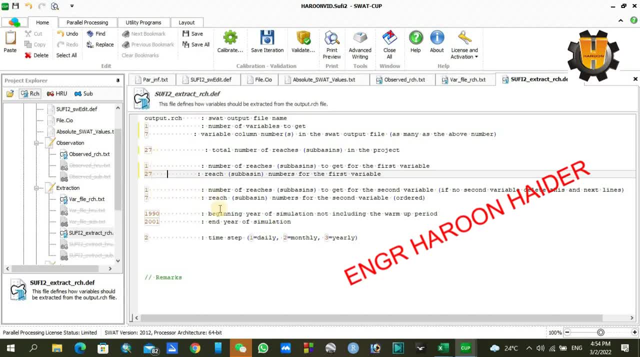 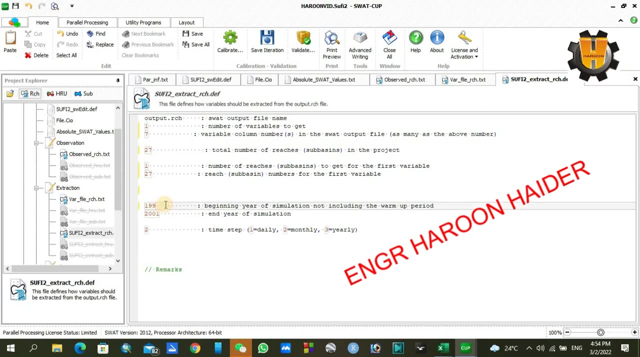 and outlet points, so 1 and 27, and number of reaches. We do not have any second variable, just delete it. So beginning year of your simulation: it should be the starting year of your project, so 1995 till 2006.. 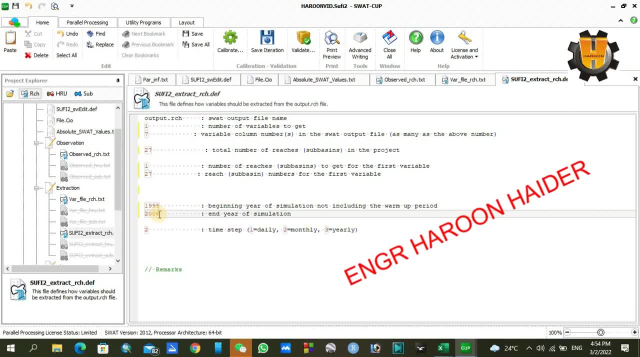 So for my calibration purposes it is 2006.. And time step: if you are using daily data, you have to paste 1 for monthly, 2 for annual, 3.. So it is already 2, so I am using monthly data. 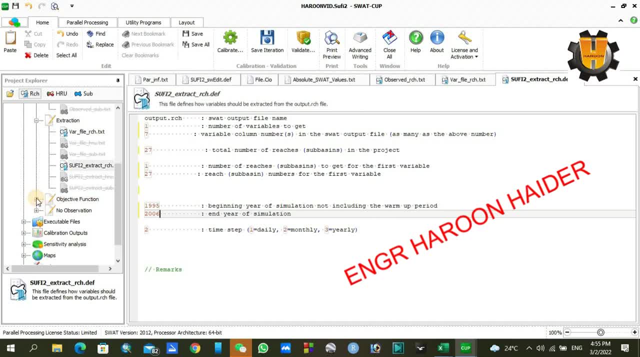 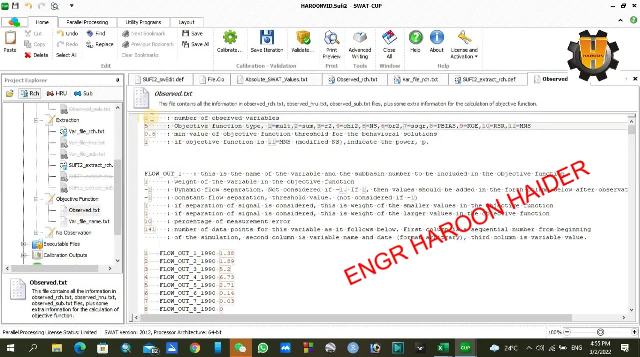 Okay again, objective function- open. objective function- observetxt- number of observed variables. we have to be 1, and objective function, so ns. okay, 5 is 5.. So we just have to change the float. it is float.7, and again you can see there are. 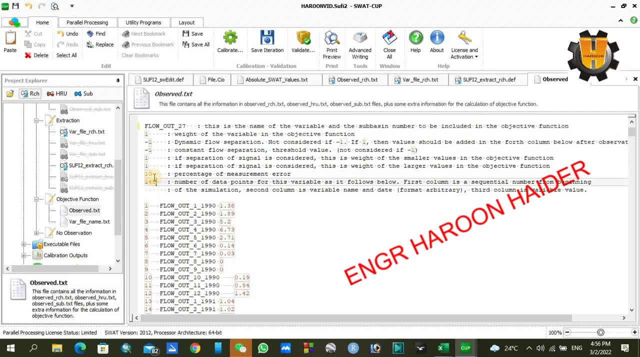 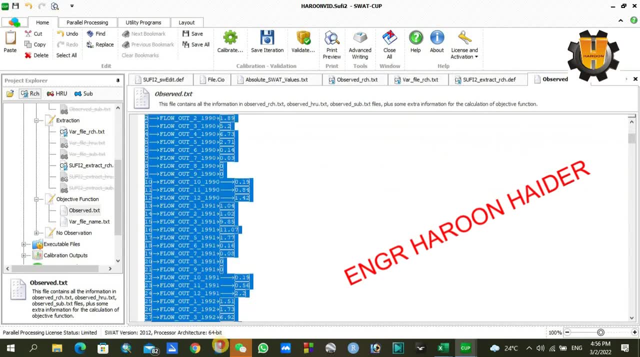 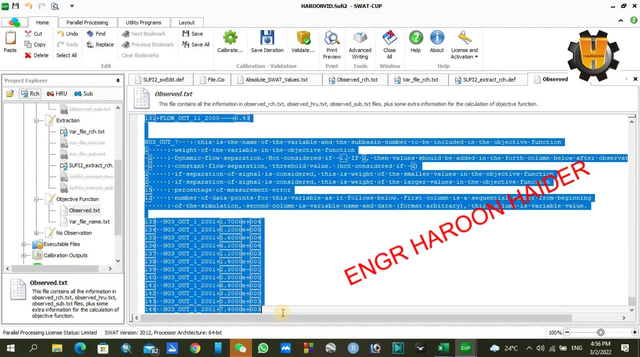 144 data points, but we have 44 here, so change this one and delete the all others. Okay, so these are the default data sets by SWAT cup. we do not need to use that. we have to paste here our data set. 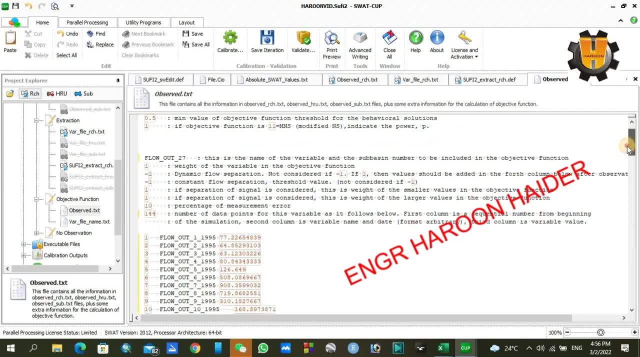 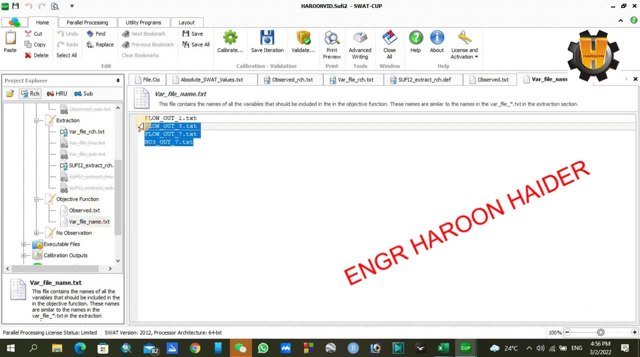 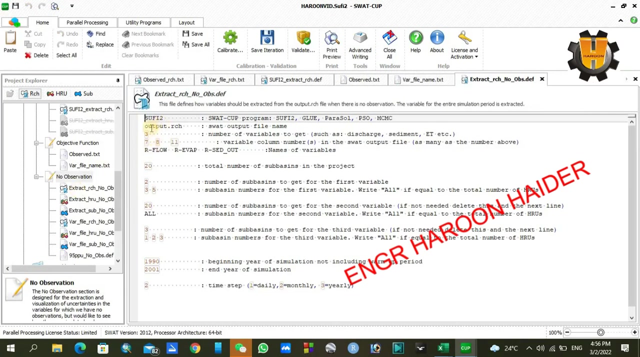 You can again copy, as I already copied it and paste it just here. okay so, variable file name. it doesn't matter which variable file name you are going to use again, I am just writing float.7.. Okay so, no observation, we do not need to change this. but again, number of variables. 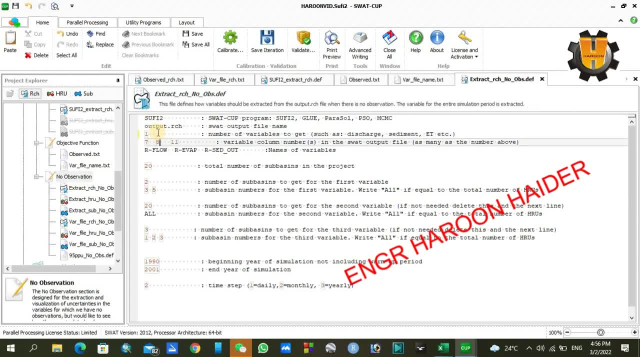 we get 1, same with float.7.. We have to be 1.. Again, we have to be down with it. And total number of submission and project 20.. We have to delete this. all, only all loadable requirements. 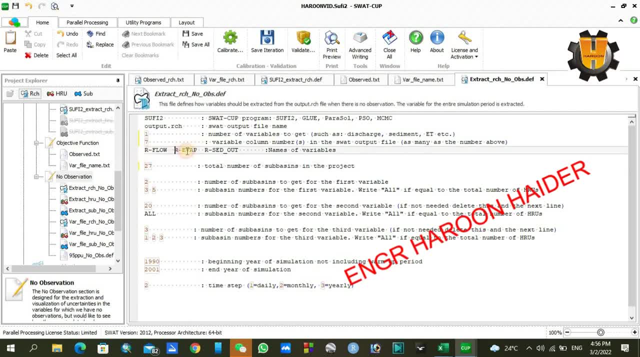 So number of submission to get for the first variable, 1, because we have only to worry about our one submission, last one. So second variable is not required. It is not required, That's it. So that's it not required. and third variable is also not for our concern. just delete it. 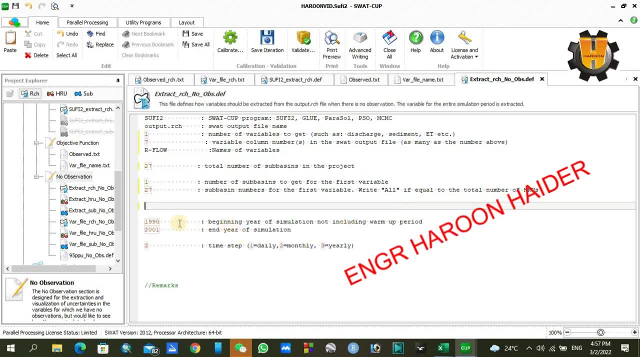 you must look at first and second variable to not delete it. ok, beginning year: as i already written, it's 1995, depending upon your project setup, and the ending year of 2006, and that is ok, so i think it's fine. so except create node. 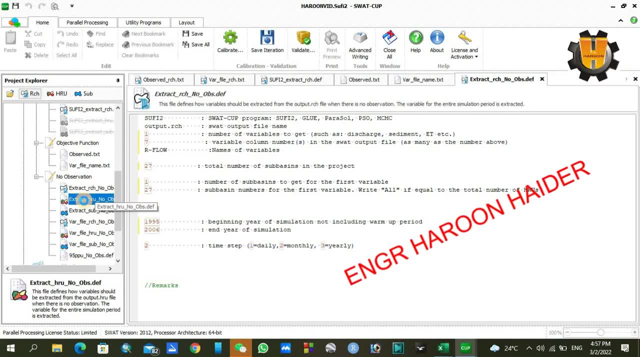 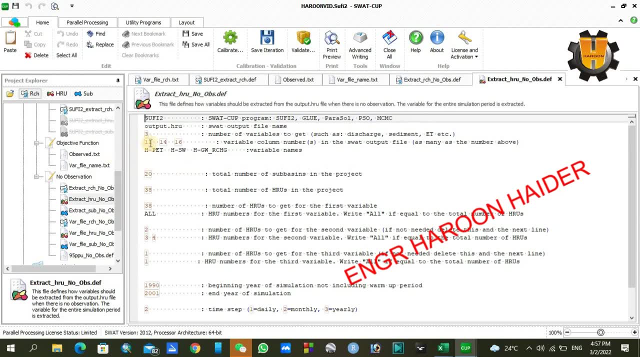 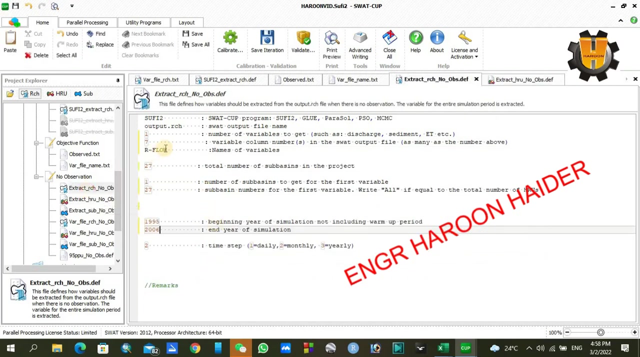 extract hreview, perhaps again make similar changes, such as: 1 variable column 7. 7 is actually the column of flow and we have to change the name and give it as our flow value here and let's create our flit, our flow, copy it. 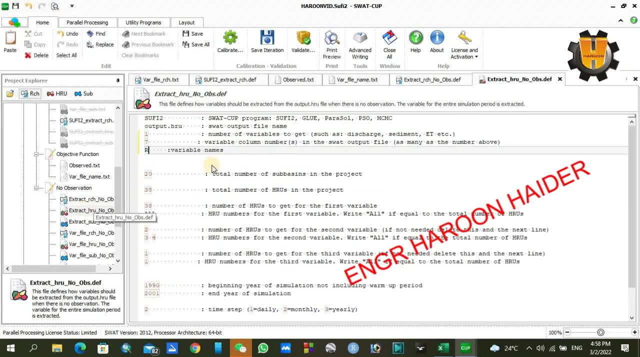 center control this. ok, so video tutorial name is done. total number of subject is 7. number of work i did is 1. number of HRU: I have 38 HRU, but one. I found one HRU, The last one because it is in last database. 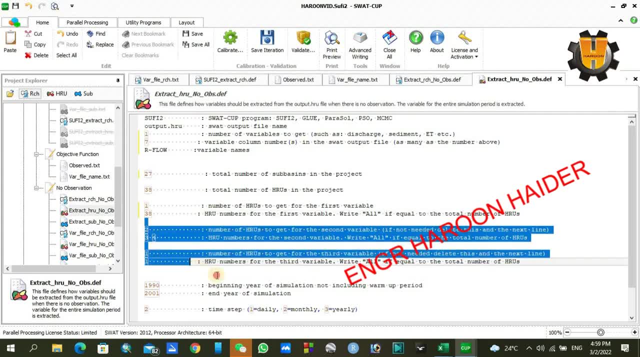 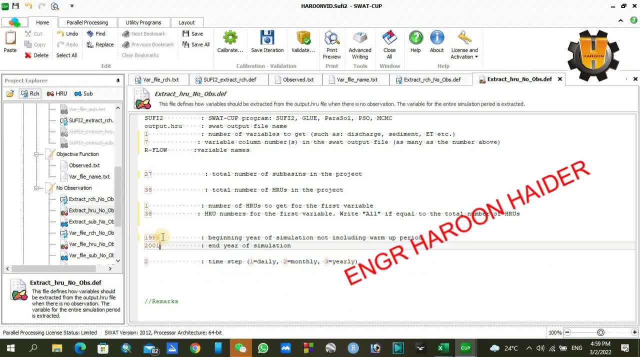 So for second variable and third variable, we do not need anything. We have to delete this And again we have to change that Beginning year is 1995 and ending year is 2096.. Okay, Similarly, we have to go for other. 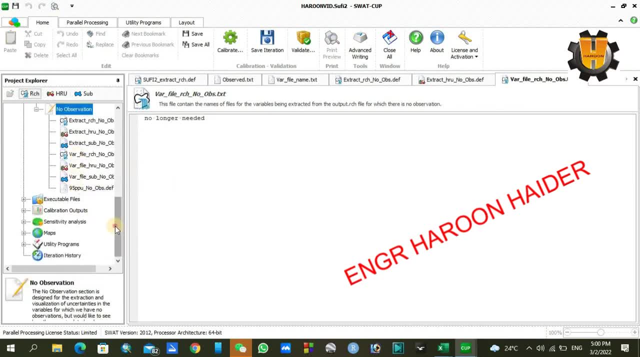 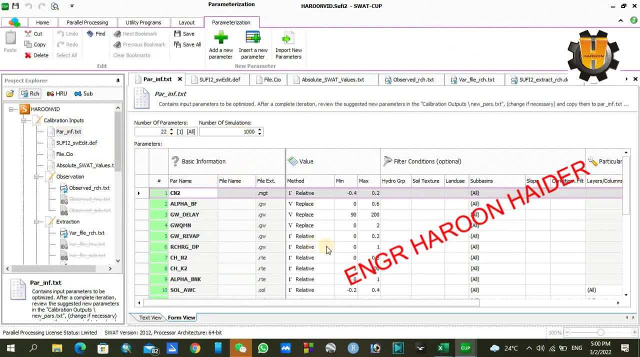 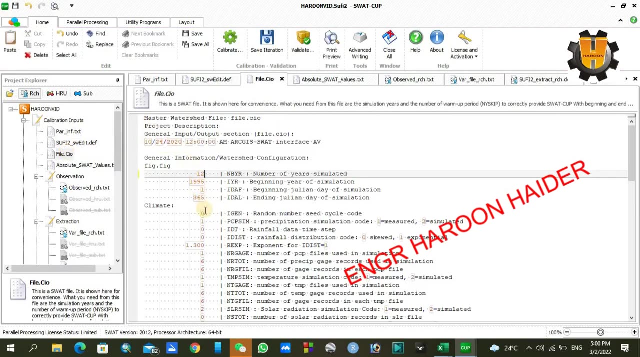 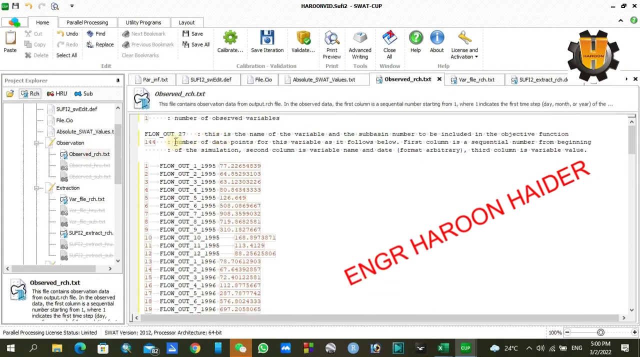 So everything is done. Then we check it: 1000 and value 1000 and 12 years- Okay, And again For second: Okay, Okay, Okay. So I think everything is fine, Just go and click on get it done. 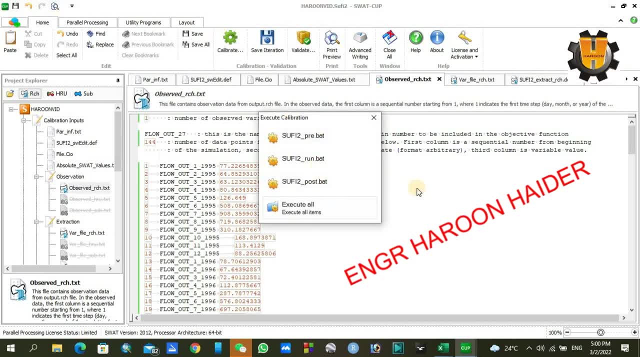 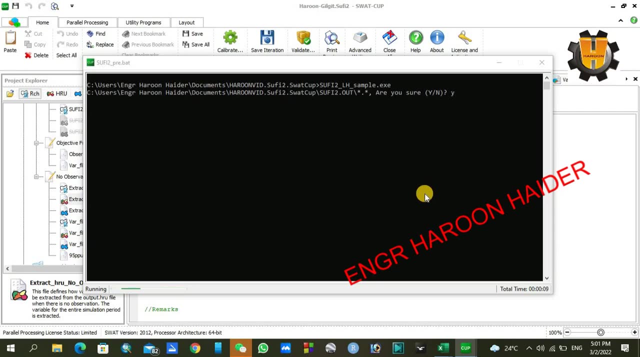 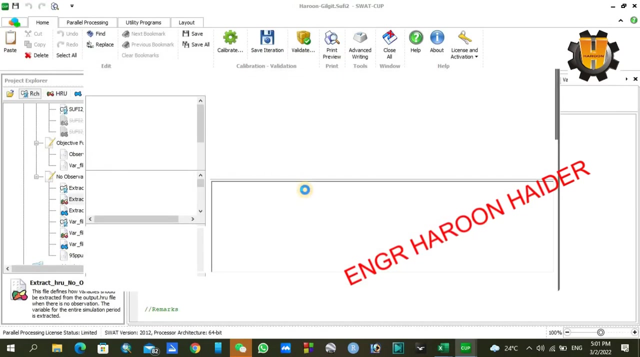 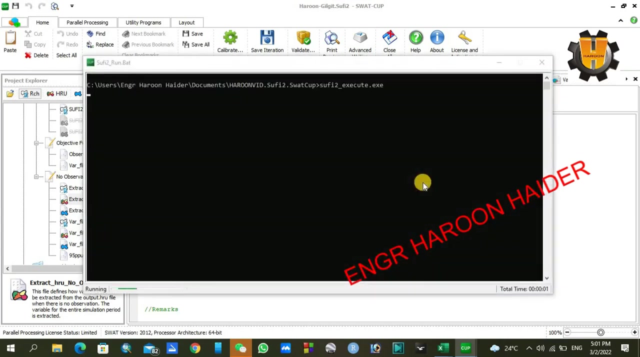 So here we have to select car item. Click on buy Car item. so let me say your organization will be started and hopefully you will get accurate results. so this process is selected. i have already run this, so let me show you my results, if you do not get any results in. 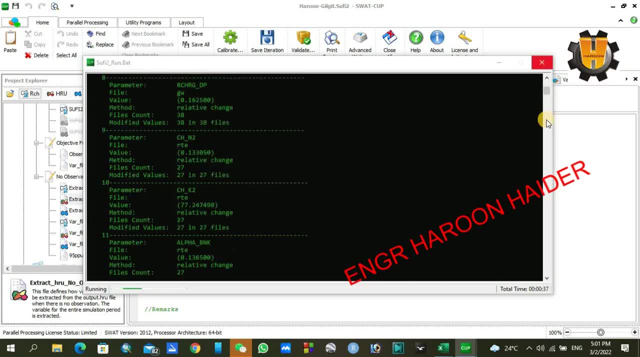 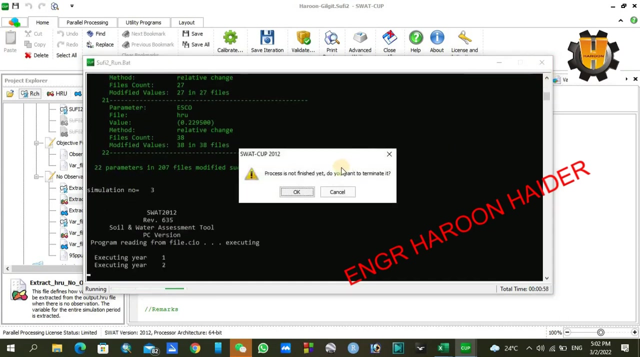 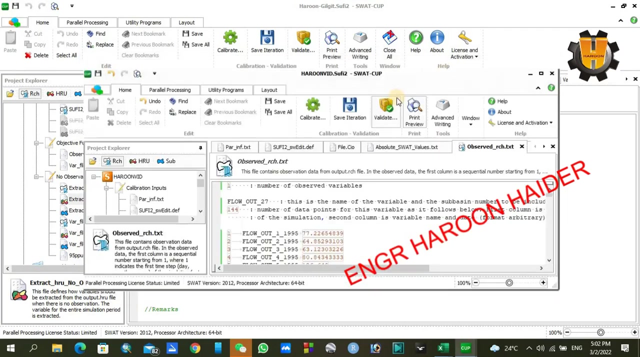 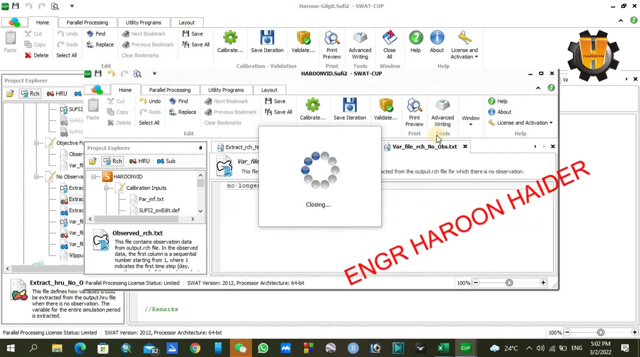 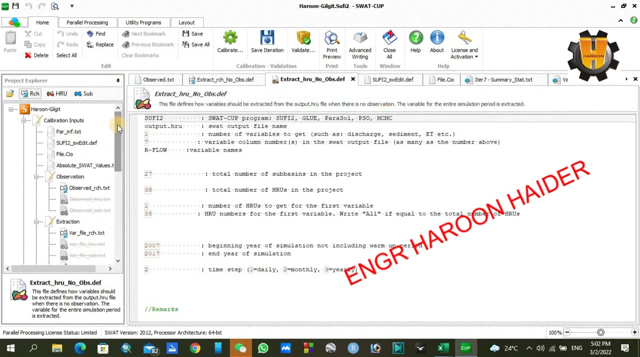 in an accurate range. you have to just replace the variables. let me show you how i have done it, because i have already run that. okay, so i'm just going to show you my results. so so this is my actual work. okay, under i question screen, i have: 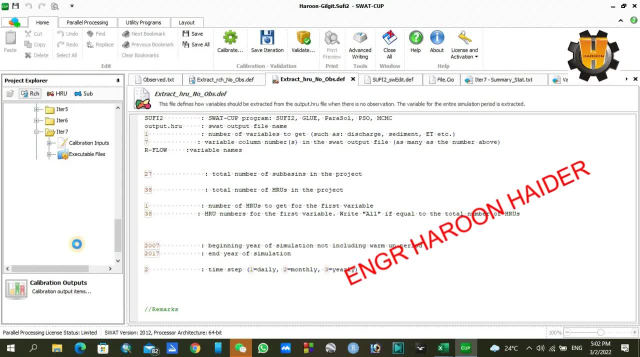 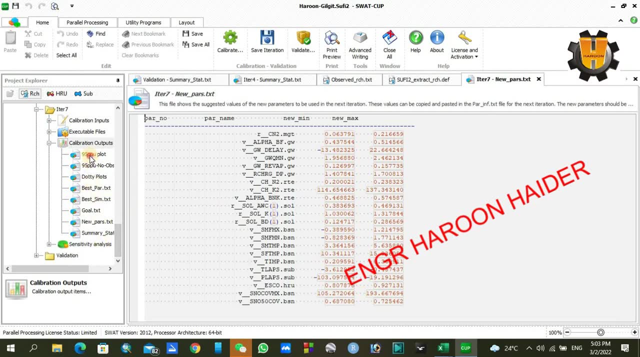 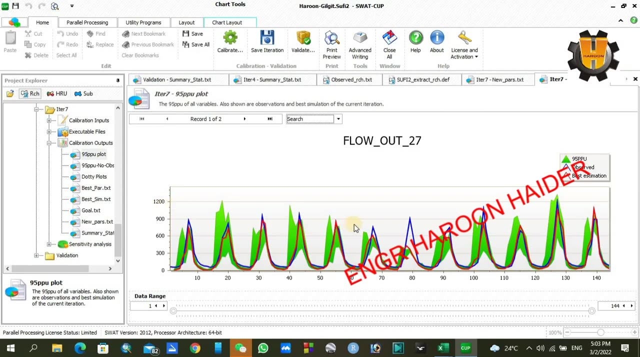 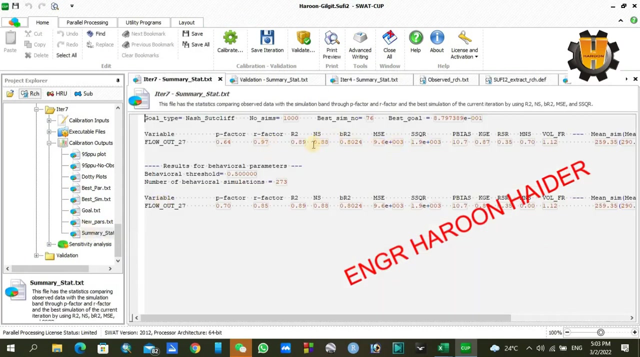 last one outputs, outputs. we have 95 pt plot. so this is the plot of my and the result of my calculation and you can see the summary also here. that is the summary. i got rck 0.89 and nasa efficiency 0.88. similarly for validation. 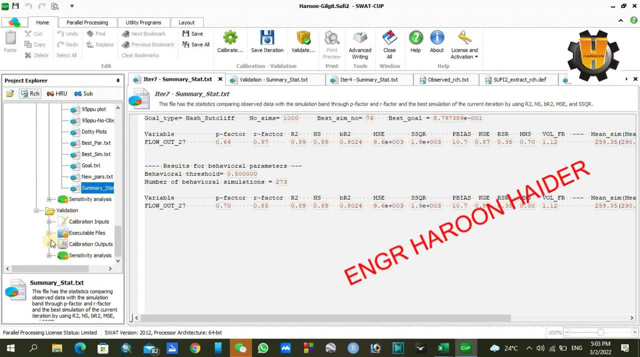 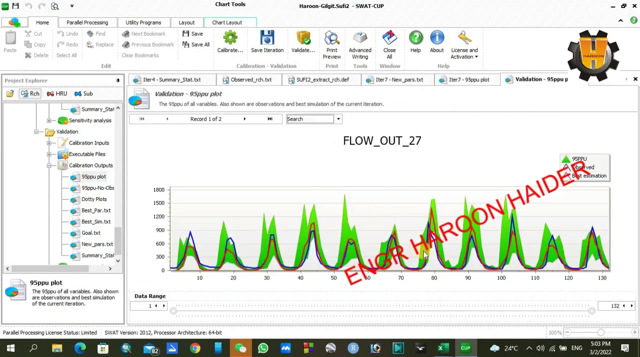 i got the outputs summary, so for my validation it is 0.82 and r square and 0.81 the ns and 95 ppu for my validation. so it's looking like this one. i hope this video will help you in the calibration work for your own. 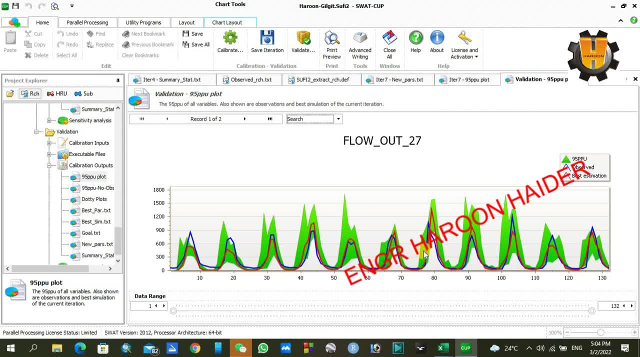 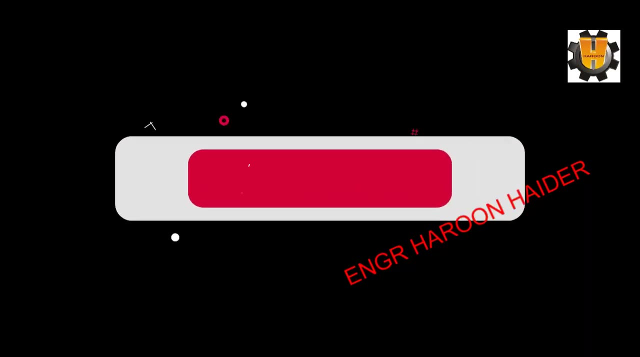 watershed. so hopefully it will help you and if you, if you, if this video is very helpful for you, then please subscribe to my channel. share it with your friends. thanks a lot, you.